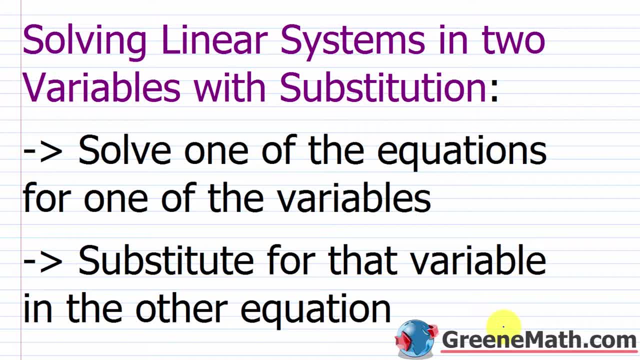 a ruler and a pencil and trying to find a solution that's, let's say, the ordered pair: 200 comma negative 400.. Okay, it's very hard to do that. It's not impossible, but it's very difficult. Or let's say, you had 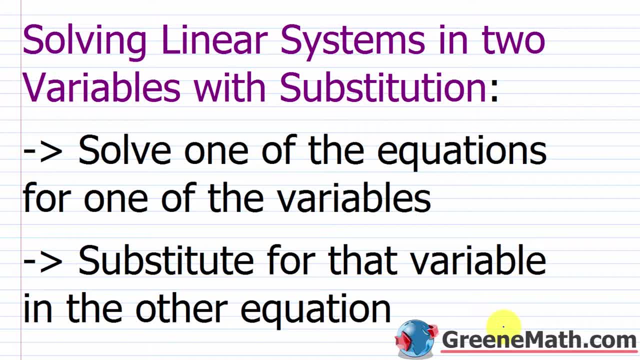 one half comma negative two fifths, Something like that. It's very hard to use graphing unless you have a small, clean, integer answer. And those were the examples that I gave, and I give them on purpose, so that you can just get a conceptual understanding. You don't want something. 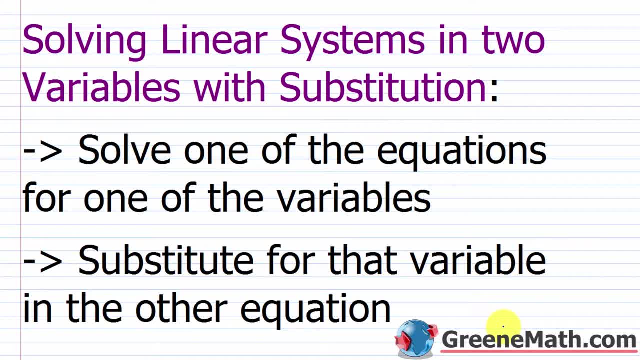 where it's just so tedious. you, you know, forget about it. I'm not going to do this. So we turn to substitution as an algebraic method. This is something you can use. no matter how big or small something is- fractions, decimals, whatever you want, you can use substitution. Now I am going to say: substitution works best when you have a 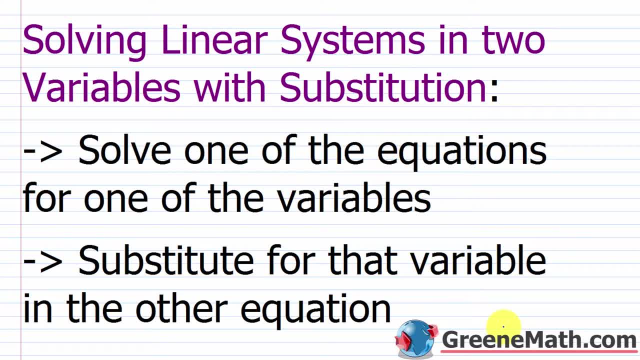 coefficient for one of the variables, that's, a one or a negative one. Okay now, with that being said, let's kind of dig into this. So solving linear systems in two variables with substitution. So the first thing that we want to do, we want to solve one of the equations for one of the 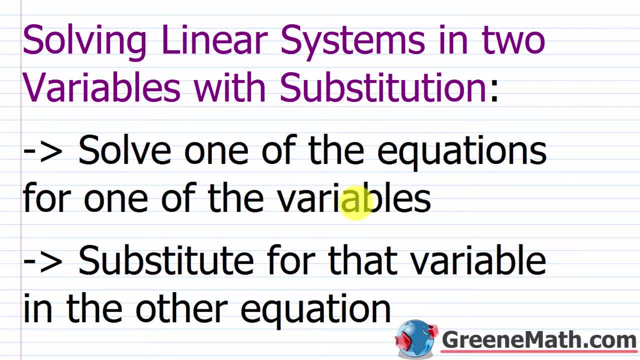 variables. So it doesn't matter which equation you use, doesn't matter which variable you start out with. Okay, it is going to be helpful, as I just mentioned, if you have a variable that has a coefficient that is one or negative one, you want to use that because it's easy to solve for that. 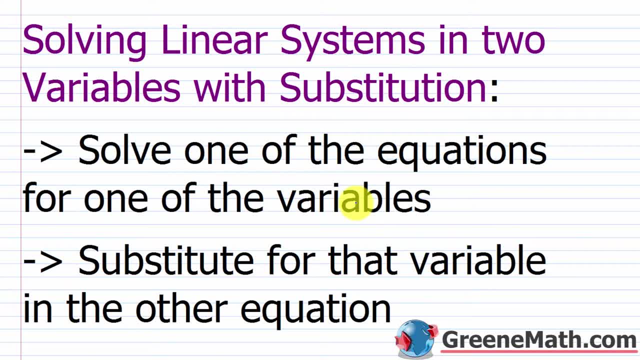 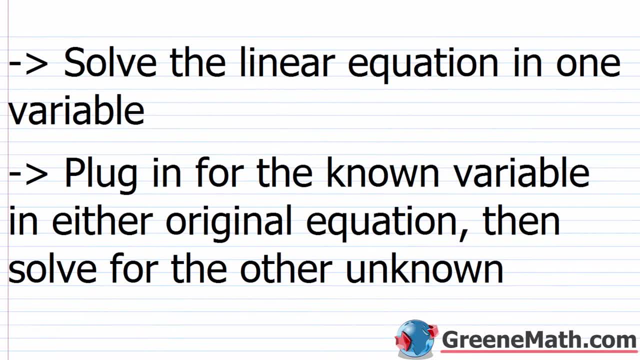 variable, But otherwise you can use whatever you want. Now, after you've done that, you want to substitute for that variable in the other equation. Now, once you finish that step, you're going to notice that that equation is going to be the one that's going to be the one that's going to be the 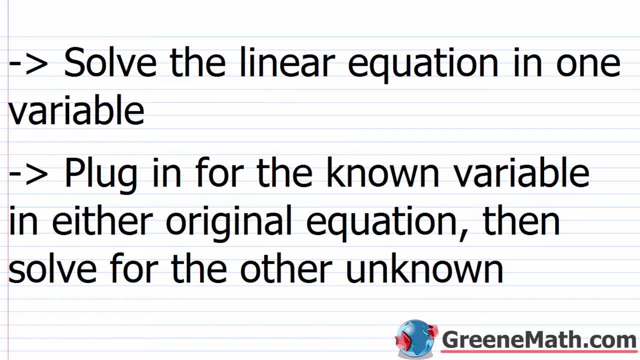 equation you're working with is a linear equation in one variable, something we've been solving forever now. So we want to solve the linear equation- one variable- and then what that is going to do is give us a solution for one of the variables. So once I have that, I plug in for the. 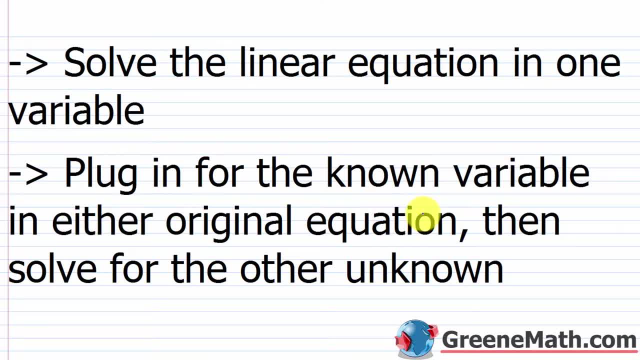 known variable in either original equation- doesn't matter which one I use- then solve for the other unknown, and I figured out the ordered pair. that is a solution for the system. And again, I say ordered pair because usually the solution is the one that's going to be, the one that's going to be. 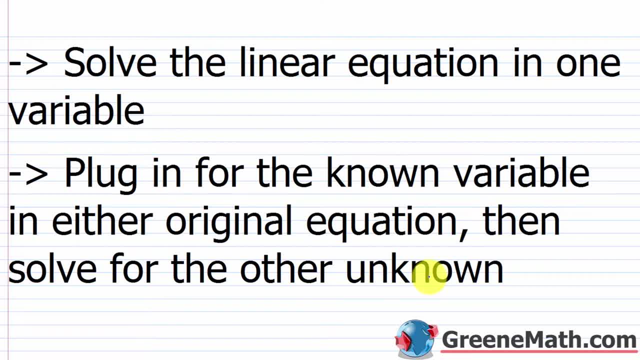 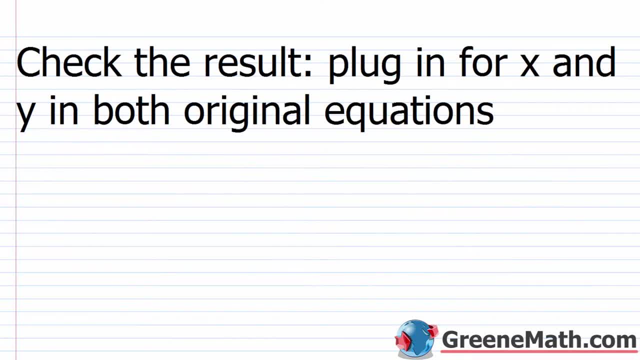 solved, because usually that's what you're going to get. You know, you have special case scenarios where you have no solution and an infinite number of solutions. I'm talking about the case where you have one solution, All right. so the last thing we want to do- and it's very important you do this- 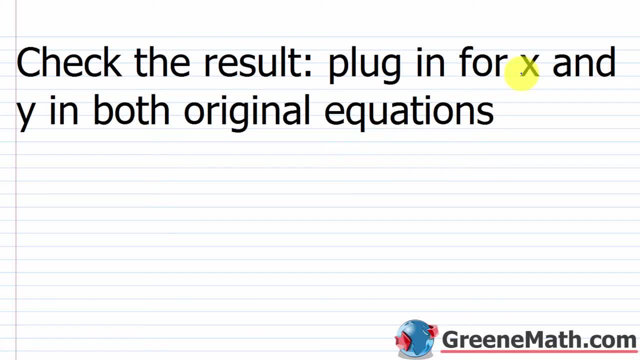 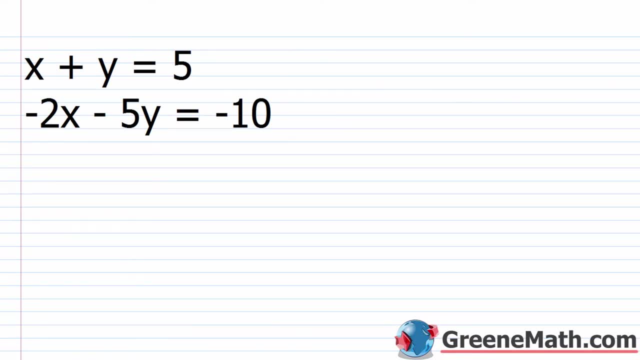 check the result. So you want to plug in for x and y in both original equations. All right, so let's take a look at the first example. So we have our linear system here in two variables. So we have x plus y equals five and we have negative two. x minus five, y equals negative ten. 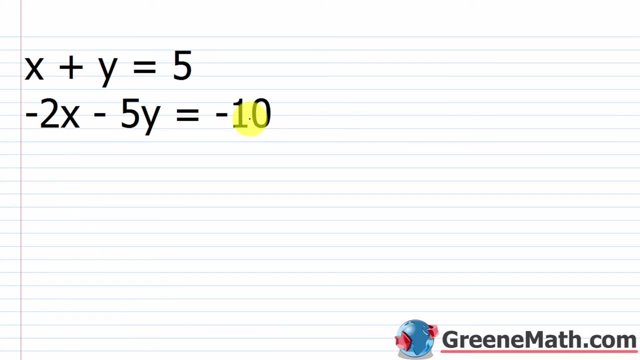 So I would pick one of the equations and solve it for one of the variables. Now, if I look at this first equation- and I'm going to label this as equation one, so I can refer to it- I'm going to label this as equation two, so I can refer to it. If I look at equation one, I notice that the 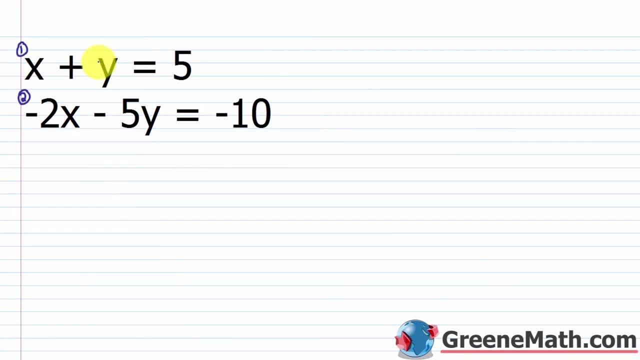 coefficient for x and the coefficient for y is a one, So it would make it pretty easy to solve for either one. So let's go ahead and just solve it for y. So if I have x plus y equals five, and I solve that for y. We've been doing this for a while now. I just subtract. 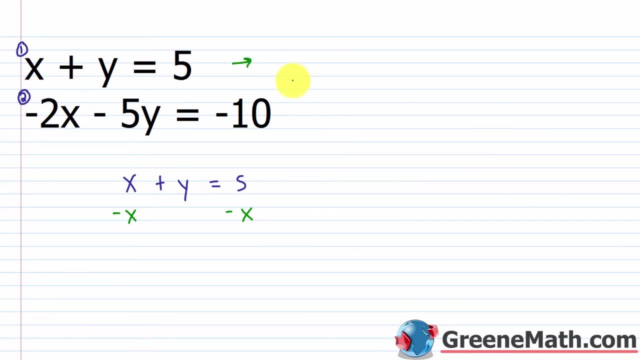 x away from each side of the equation, and so this would become: y is equal to. I'd have negative x plus five. Now I want you to think for a second what the equals sign means Equals is saying is the same as. So y is the same as negative x plus five. 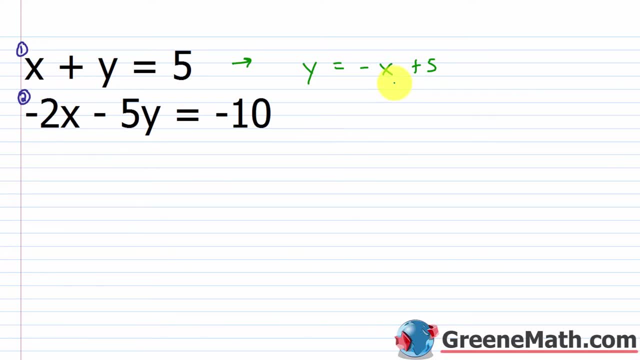 It's like if I have money and I say a dollar is the same as four quarters, They are the same in value. They don't look the same, but they are the same. If I give a cashier four quarters, If I give a cashier a dollar bill, I've presented the same value to the cashier and so that is one dollar. 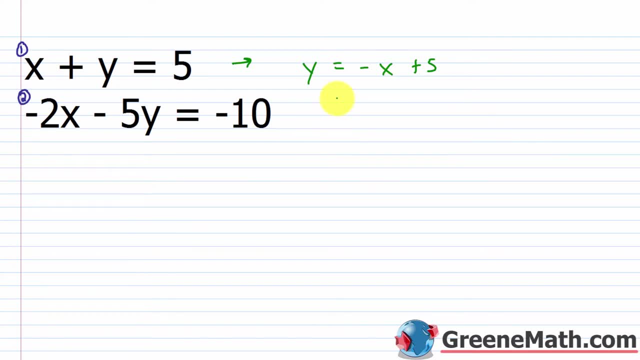 either way, Okay. so now that we have solved this guy for y, I am going to plug into the other equation. Okay, so I'm going to plug in for y here Again. y equals this, So this is going to get plugged in there. It's all I'm doing, So I would. 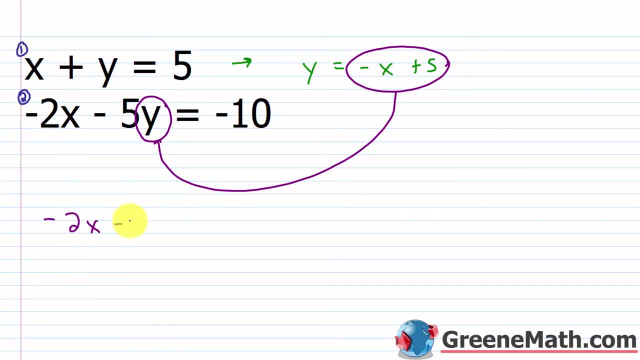 have what In equation? two negative two x minus five. I've got to use parentheses here, because five is multiplied by y and y. is this: Y is the quantity negative x plus five And this equals negative ten. So notice that I have substituted in for y in the second equation. 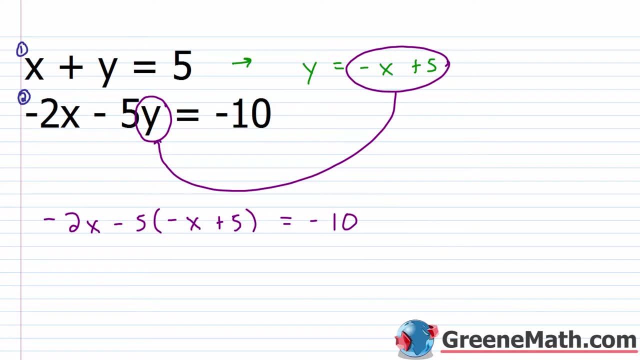 And the result here is a linear equation in one variable. I now only have to deal with x, and that's pretty easy to do. So I have negative two x. I have negative five times negative x, That's plus five x. And then negative five times five is minus twenty five, And this equals negative ten. 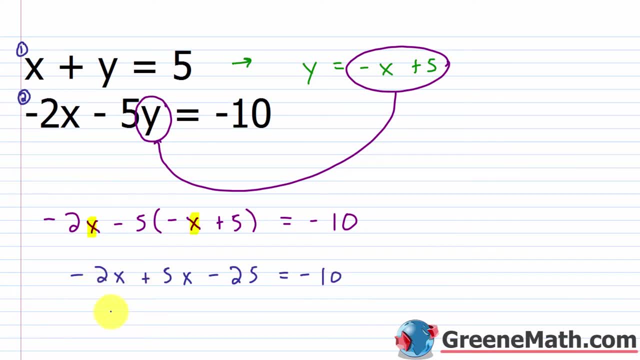 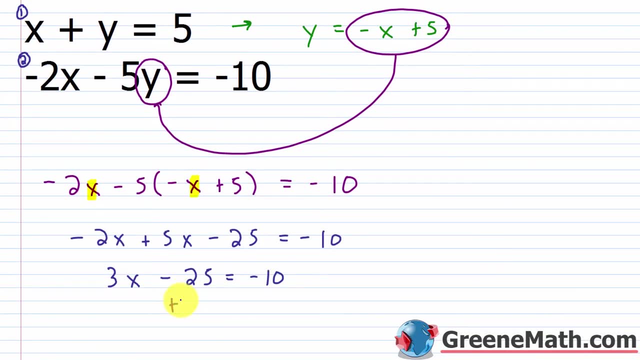 Combine like terms on the left: Negative two x plus five x is three x And minus twenty five equals negative ten. Let's go ahead and add twenty five to y And then I'm going to plug in each side of the equation. This will cancel. We'll have three x is equal to negative ten plus. 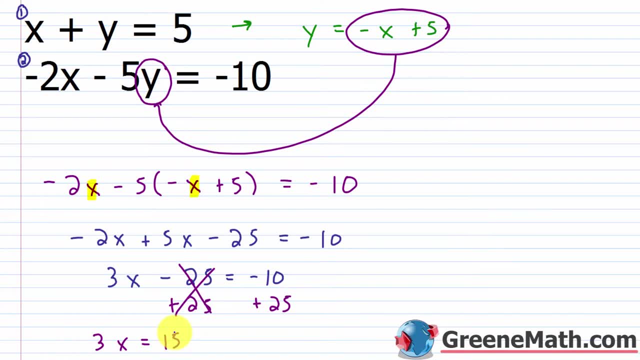 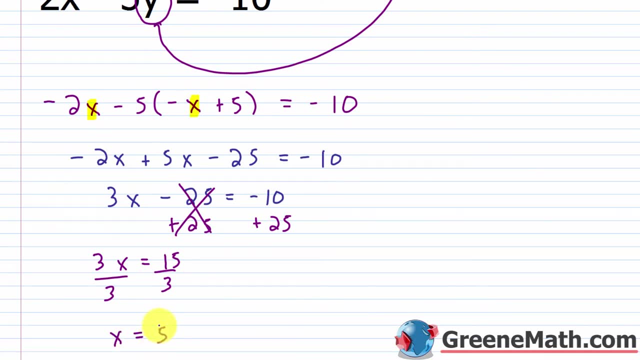 twenty five is fifteen. Let's scroll down and get a little room going. We divide both sides by three and we get x is equal to five. Now for the ordered pair. that is my solution to the system. I already know that x is five. Let me erase everything I've done to this point. So we know x is five. 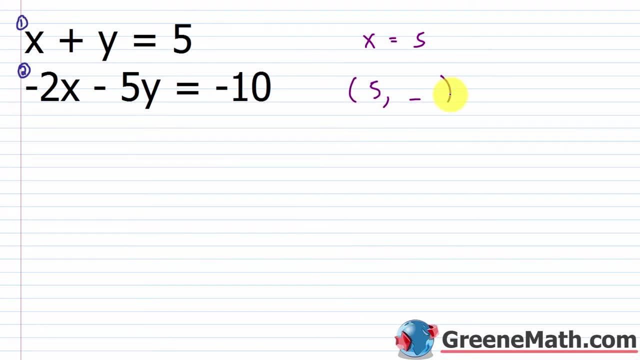 So for the ordered pair I'd have five comma something. Now how am I going to get this other something? Well, five works as a solution for x in both equations if it's a solution for the system. So I can plug a five in for x here in equation one or here in equation two and solve for the. 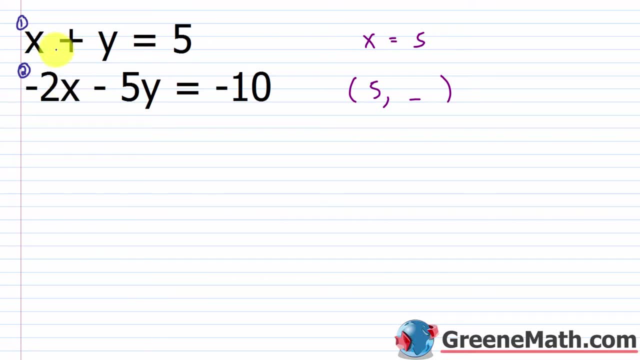 unknown y. So let's go ahead and do it in equation one, because it's a much simpler equation. So we would have five plus y equals five. Well, we know y equals five. So we know y equals five. So we can go through the steps: Subtract five away from each side of the equation. This will cancel. 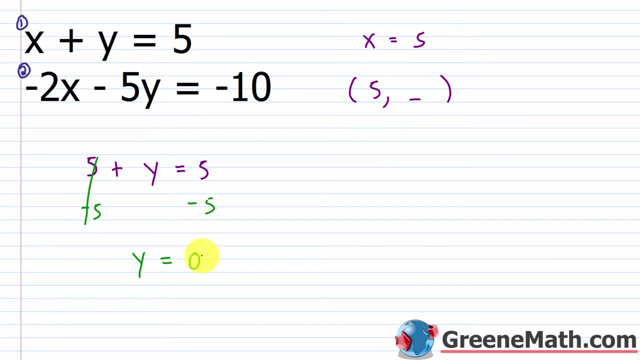 You'll get: y is equal to five minus five is zero. So five comma zero. Now again, I want to check this to make sure that my answer is correct. So let's erase everything. We have: x plus y equals five. So x is five plus y is zero equals five. We know that's true. Five equals five. We just did that. 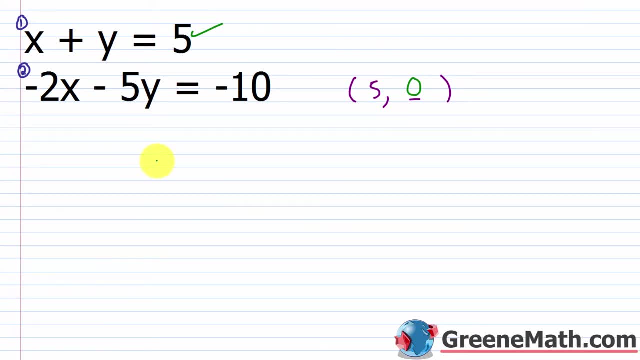 The other one, you would have negative two. So negative two times plug in a five for x minus five times plug in a zero for y equals negative ten. Negative two times five is negative ten. Of course. negative five times zero is zero. So I get negative ten equals negative ten. So that's. 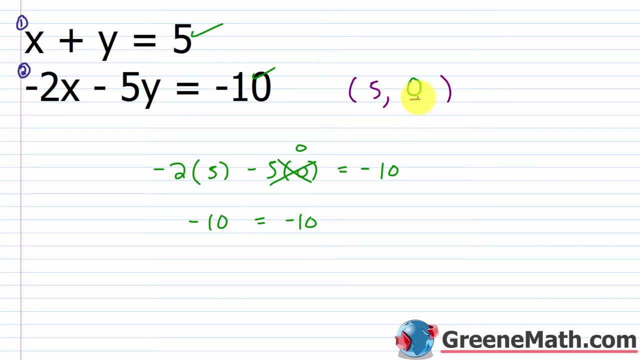 true as well. So we verified that the ordered pair five comma zero is the solution for this system. What if I would have- let me just let me just Throw this out here- What if I would have chosen equation two to start out with? And let's say: 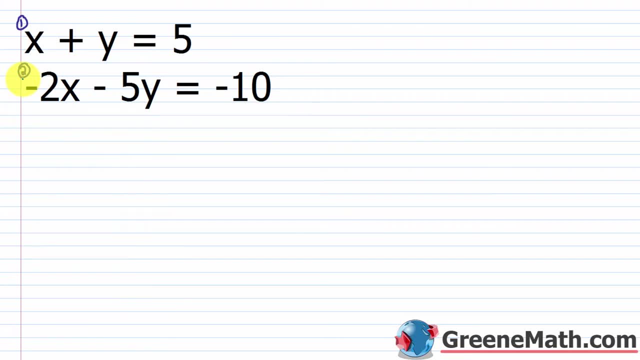 instead of solving for y, I solved for x. Would I get the same answer? The answer to that is yes, Let's go ahead and do that. So I have negative two x minus five y equals negative ten. So I'm going to solve for x. So I'm going to add five y to both sides of the equation. So this will cancel. 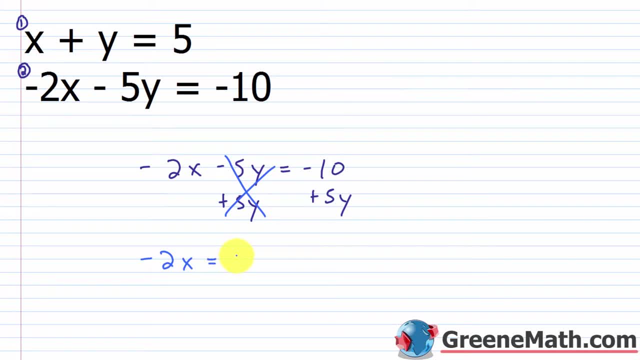 I'll have negative two. x is equal to. You'll have y minus ten. And then let's go ahead and divide both sides of the equation by negative two. So this is going to cancel. I'll have x is equal to five over negative two. Might as well, just put. 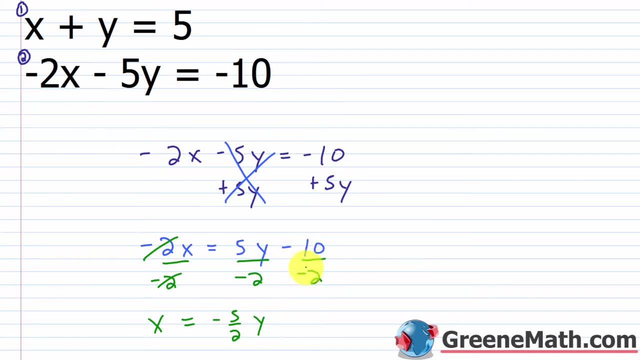 negative five halves times y. Negative ten over negative two is plus five. So this came from equation two. So I want to plug into equation one. And what do I want to plug in? for I know that x equals, x equals this value. 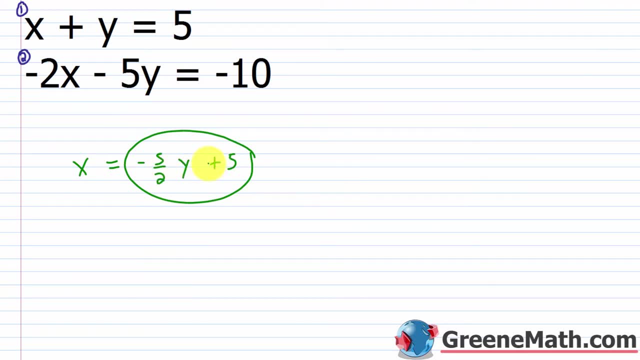 Negative five halves y plus five. So x is the same as that. So I'm going to plug in for x in this equation now And I'm going to plug this in. So when I do that, what happens? I have negative five halves y plus five. Then plus y equals five. So now I have a linear equation in one variable. 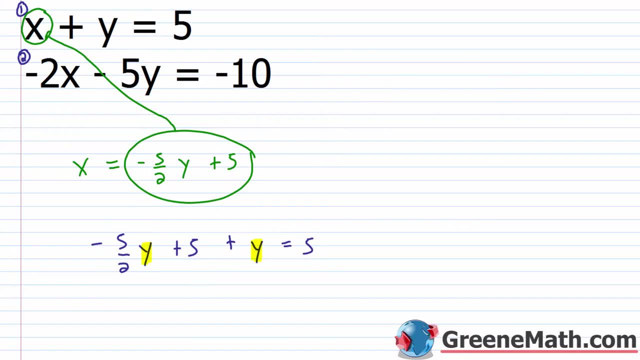 I just have a variable y, And again that's very easy to solve for. So if I subtract five away from each side of the equation, this will cancel, and this will cancel. You'll have negative. five. halves y plus y equals zero. Now, before I do anything else, you know that the 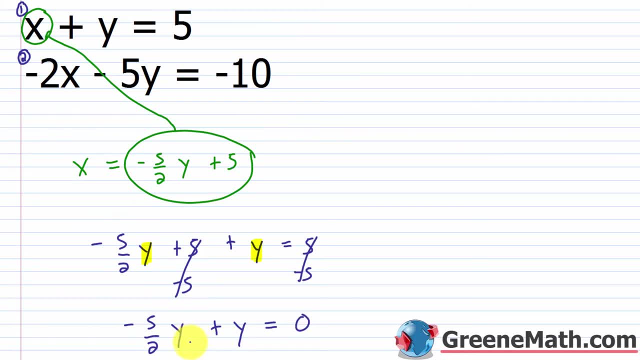 answer for y was zero, And you can see that the answer for y would be zero here. No matter what, when I combine like terms, I'm going to have something: times y equals zero. That can only be true if y is zero, So you don't need to go any further. You've proved it to yourself. But for the 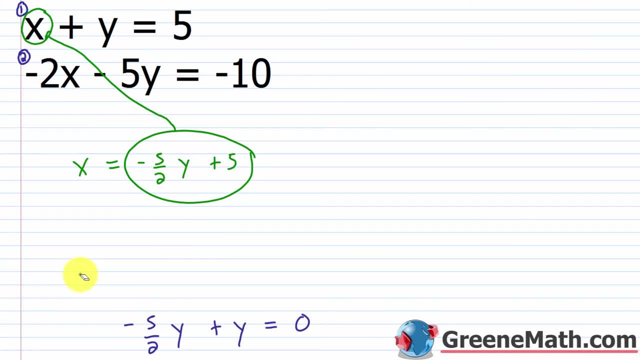 greatness, I'm going to go all the way here. So let me bring this up And let's go ahead and just multiply both sides of the equation by two. That'll be the easiest way to do this. So two times negative five halves is negative five times y. Two times y is plus two y And this equals zero times two. 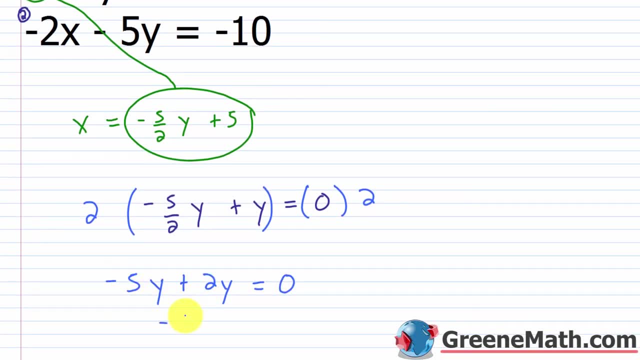 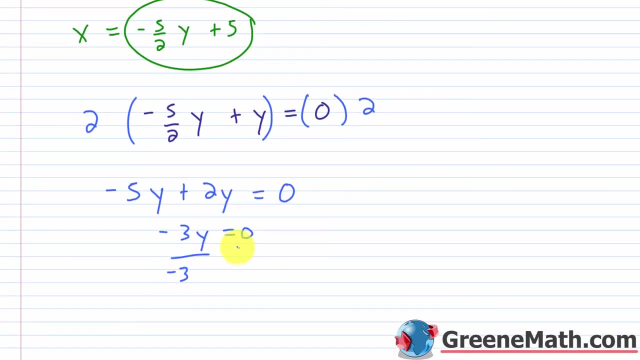 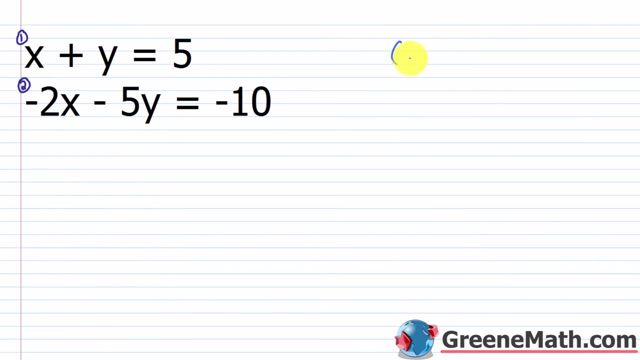 which is zero. So negative five y plus two y is negative three y And this equals zero. And of course we know that y equals zero. So what is x? Again, plug in for y in either original equation. I can plug into this one or this one, Doesn't matter, Let's go ahead and use the second one. 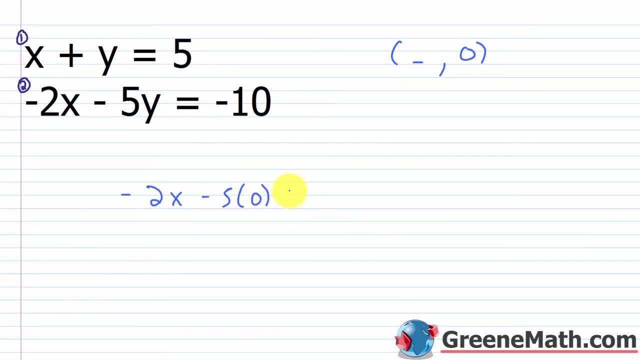 So negative two x minus five times zero equals negative 10.. So this will go away. I'll just have negative two. x is equal to negative 10.. And then I'm going to plug in for y in either original equation: Negative 10, divide both sides by negative two, So this will cancel Negative 10 over negative two. 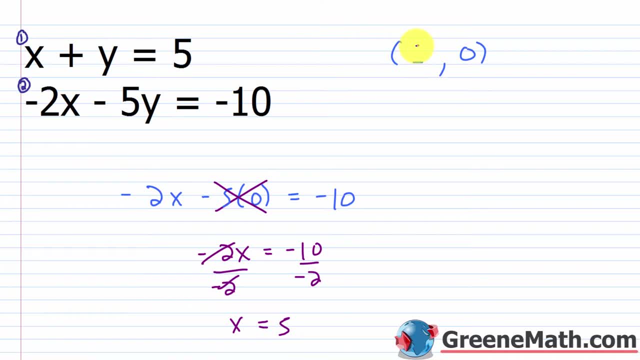 is five, So you'll have: x is equal to five, So I get five comma zero as the ordered pair, as we already found. So any way you do it, you can solve for any variable in any equation to start And you're going to plug in for that variable in the other equation. All right, for the next one. 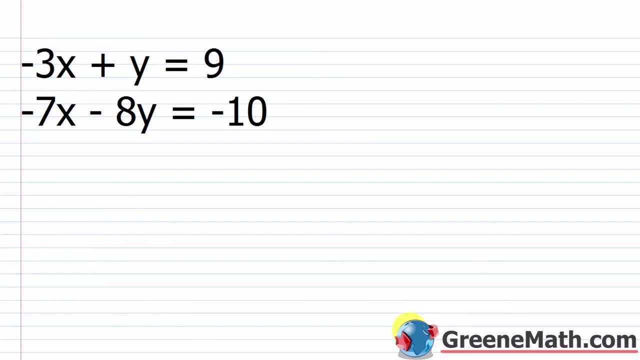 we have negative three: x plus y equals nine. And we have negative seven: x minus eight, y equals negative 10.. And we're going to plug in for that variable in the other equation. And we're going to plug in for that variable in the other equation. And we're going to plug in for that variable in the other equation. 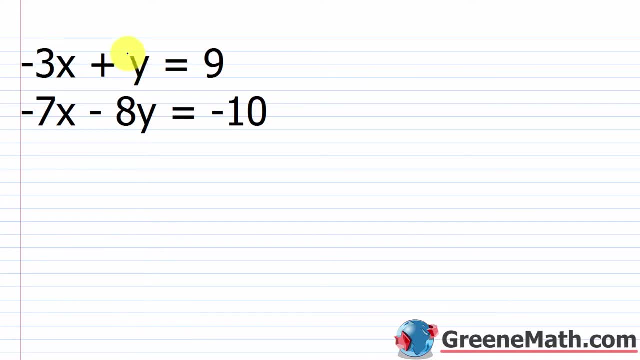 So the first thing I want you to notice here is that you have a coefficient of one when you're a variable y in. what I would like to say is the first equation, So I'm going to label this as equation one. This is equation two. Just for reference sake, I say, hey, equation one, I'm talking about this one. 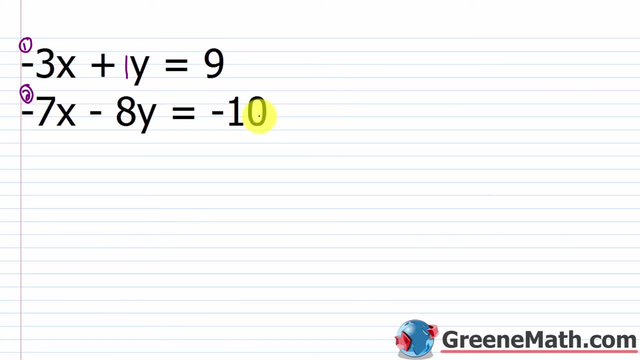 Equation two. I'm talking about this one. So the easiest thing to do here, since I have a coefficient of one there, is to solve equation one for y. So let's go ahead and do that. Let's say that we have negative three x plus one, And we're going to plug in for that variable in the other equation And we're going to 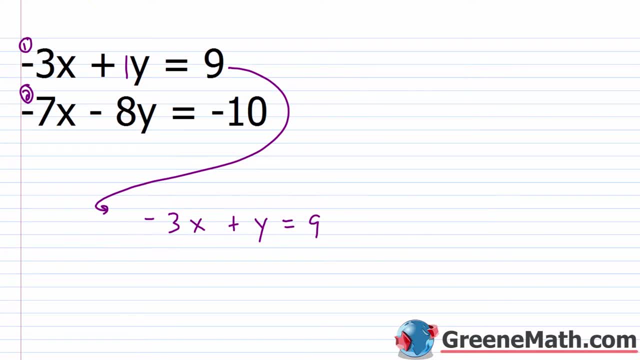 plug in for that variable in the other equation. So let's say that we have negative three x plus y equals nine. All I've got to do is add three x to both sides of the equation And this will cancel. I'll have: y is equal to three x plus nine. So that's super simple. All right, now that I know what y is equal to or what y is the same as, I can plug in for y in the other equation. So I'm going to plug this again: what y is equal to, or what y is the same as in for y, And I'm going to plug this in for y in the other equation. So I'm going to plug this again: what y is equal to, or what y is the same as in for y, And I'm going to plug this again. what y is equal to, or what y is the same as in for y, And I'm going to plug this again: what y is equal to or what y is the same as in for y, And I'm going to plug this again. 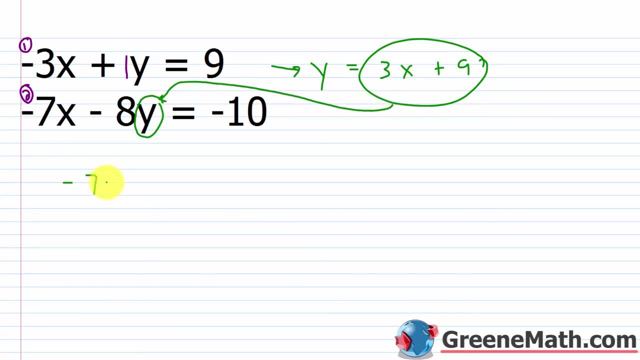 this. So I would have negative 7x minus 8 times. Again, it's this whole quantity that y is equal to, So 8 is multiplied by that quantity. So I'm going to use parentheses: 8 times the quantity 3x plus 9. And this equals negative 10.. So let's go ahead and solve this equation for x, You'll 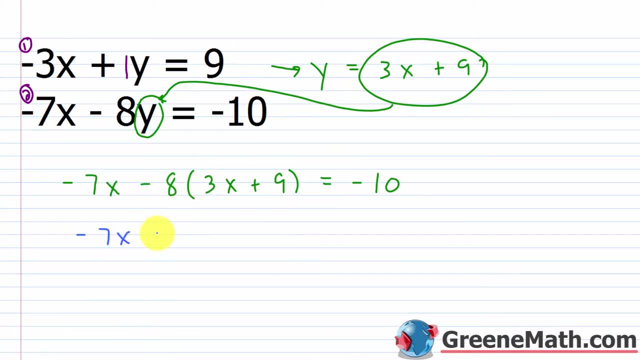 have negative 7x And then you have negative 8 times 3x. That's negative 24x. Negative 8 times 9 is minus 72. And this equals negative 10.. So negative 7x minus 24x is negative 31x. So you'll. 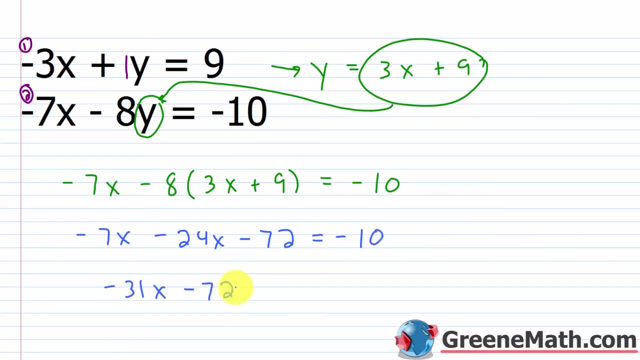 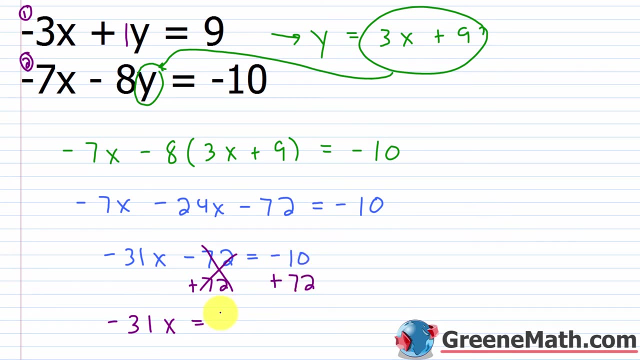 have negative 31x minus 72 equals negative 10.. So let's go ahead and add 72 to each side of the equation. That'll cancel. You'll have negative 31x is equal to negative 10 plus 72 is 62. So as a 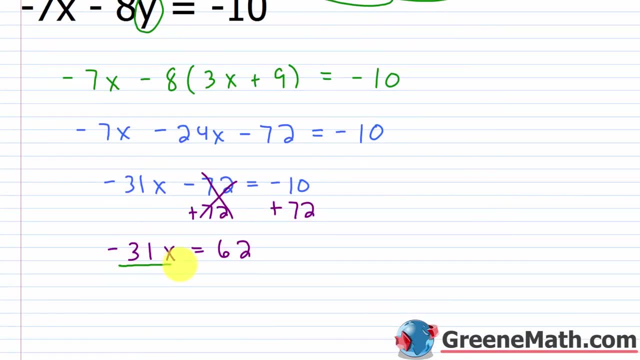 last step: to get x by itself, you're going to have to add 72 to each side of the equation. Let's divide both sides by negative 31.. This will cancel And we'll see that x is equal to negative 2.. So let's go ahead and erase everything. So we already know that x is equal to negative 2,. 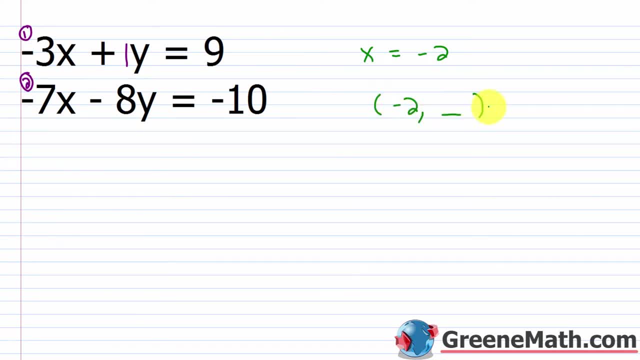 whereas an ordered pair would be negative 2 comma and then something. So I can plug a negative 2 in for x in either original equation. It doesn't matter, because in terms of the system I know x is equal to negative 2.. So this one's easier to do in equations. 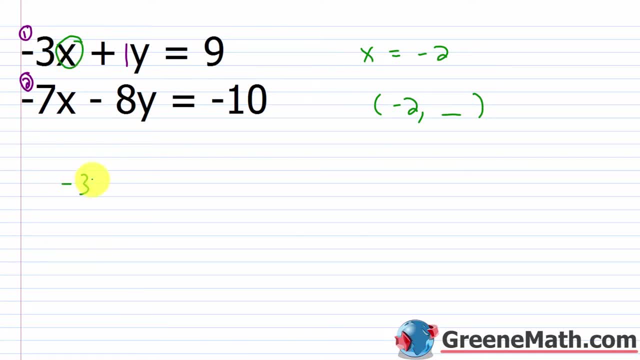 Let's just use that. So you would have negative 3 times negative. 2 plus y is equal to 9.. So negative 3 times negative 2 is 6.. So you'd have 6 plus y equals 9.. Subtract 6 away from each side of. 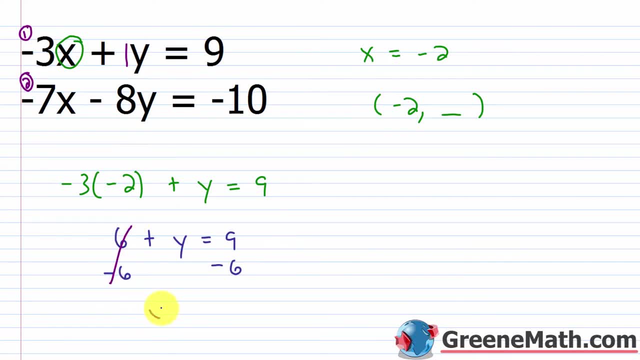 the equation And this will cancel, We'll have: y is equal to 9 minus 6 is 3.. So my ordered pair is negative, 2 comma 3.. Let's erase all this. And so now we just want to check, We want to. 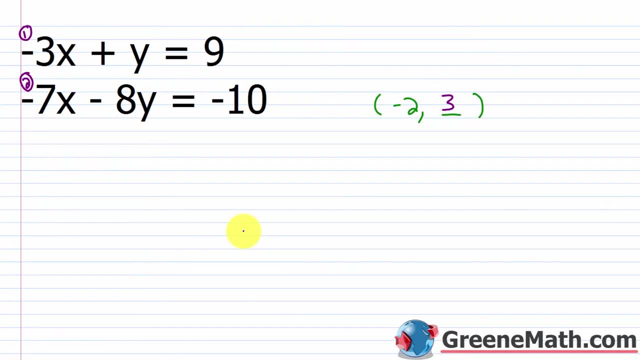 check an x value of negative 2 and a y value of 3 in each original equation. So I'm going to start with equation 1.. I'd have negative 3 times x. x is negative 2, plus for y I have 3.. And this should. 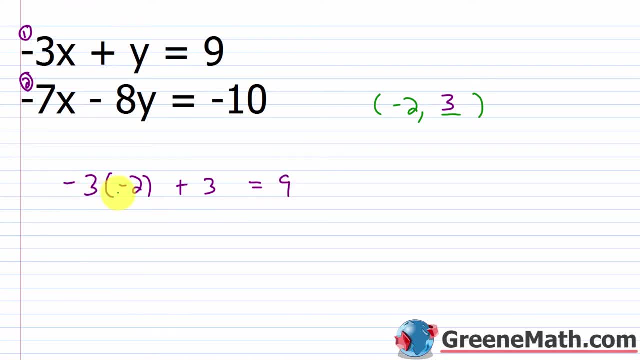 equal 9.. We know this works because we just did it. Negative 3 times negative, 2 is 6.. 6 plus 3 is 9.. So you get 9 equals 9.. So this works out there All right. For equation 2, we have negative 7. 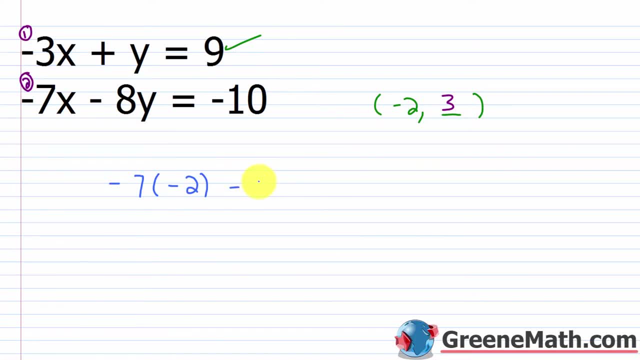 times x: Again x is negative 2.. Then minus 8 times y, which is 3.. And this should equal negative 10.. Negative 7 times negative 2 is 14.. Negative 8 times 3 is negative 24.. And again this should equal negative 10.. And it does. 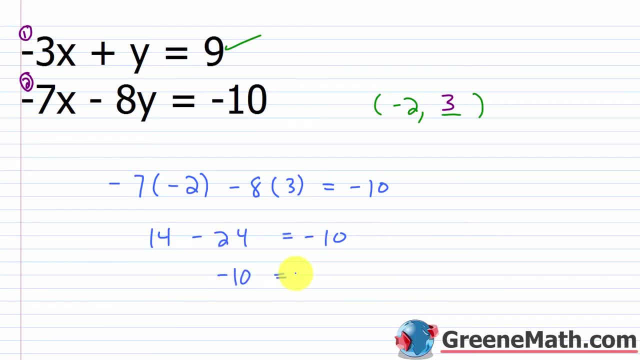 right: 14 minus 24 is negative 10. So you get negative 10 equals negative 10. So you can check this one off as well. So the ordered pair: negative 2, comma 3, or an x value of negative 2,. 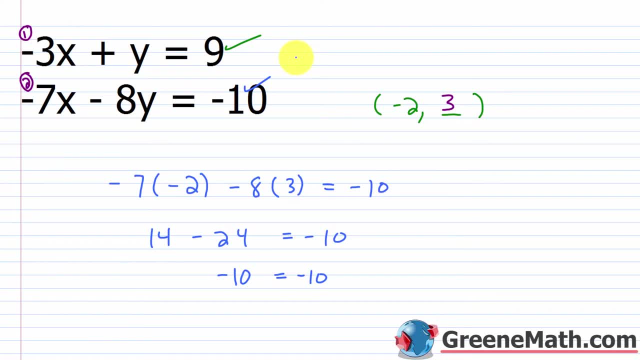 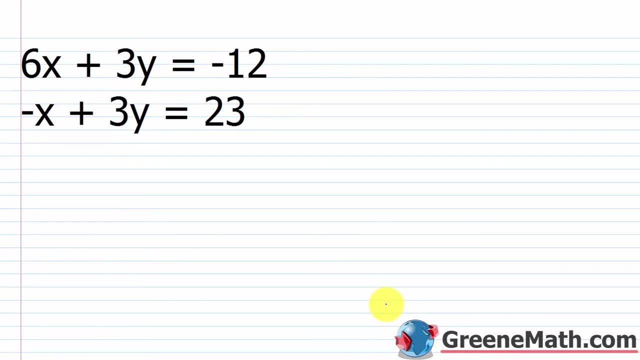 a y value of 3, is the verified solution for this system. All right, Let's take a look at another one. So we have 6x plus 3y equals negative 12. We have negative x plus 3y equals 23.. So again, if I find a variable in my system that has a coefficient of 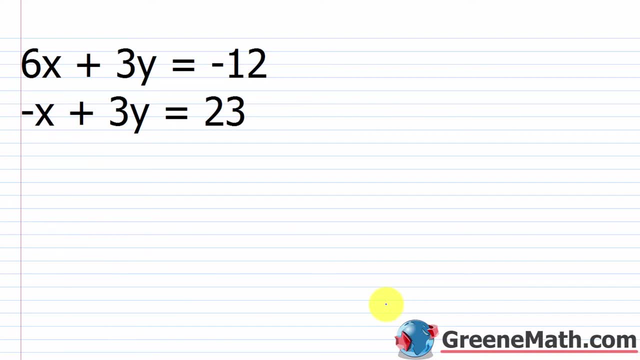 1 or negative 1, I want to use that as what I solve for. So here again, with negative 1 being there, I'm going to start out by looking at that. So, again, I'm going to label this as equation 1.. 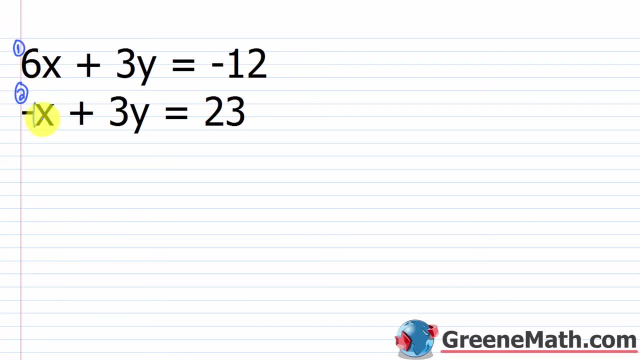 This is equation 2.. So with equation 2, I'm going to solve it for x. So I have negative. x plus 3y equals 23.. And a couple of things I can do here. I can swap sides with this one and this one, Or I can just move 3y over and multiply both sides by negative. 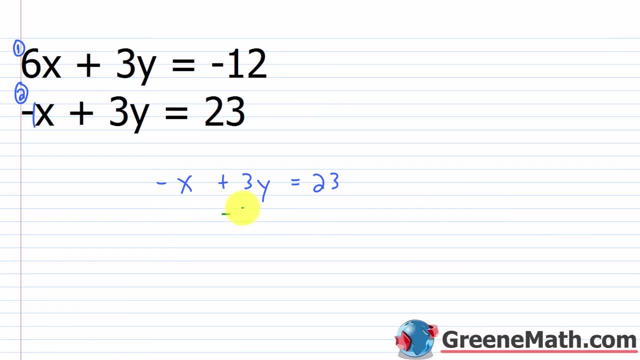 1,. whatever you want to do Doesn't matter, So let me just subtract 3y away from each side of the equation. That's how I'd like to do it. I'll have: negative x is equal to negative 3y plus 23.. 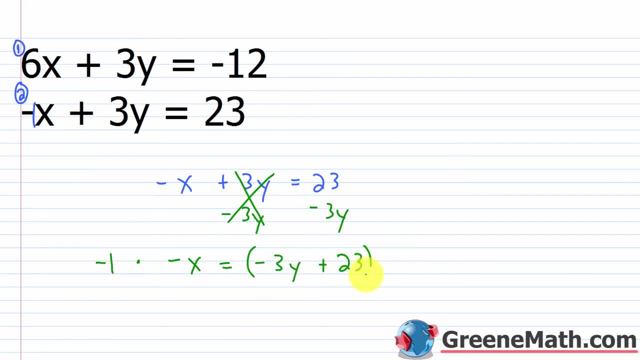 And let me just multiply Both sides by negative 1.. So negative 1 times negative, x is of course x, And this equals negative 1 times negative. 3y is 3y. Negative 1 times 23 is minus 23.. So I've solved this guy. 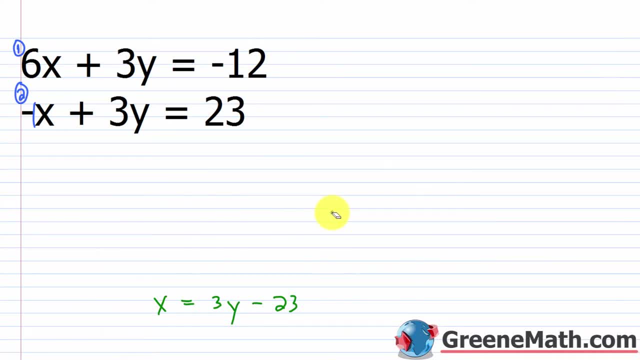 for x. So let me erase this. I'm going to drag this up And if I've solved this for x, I can plug in for x in equation 1.. So I would have 6 times The quantity 3y minus 23.. Again, x is equal to, or x is the same as 3y minus 23.. So I can plug in. 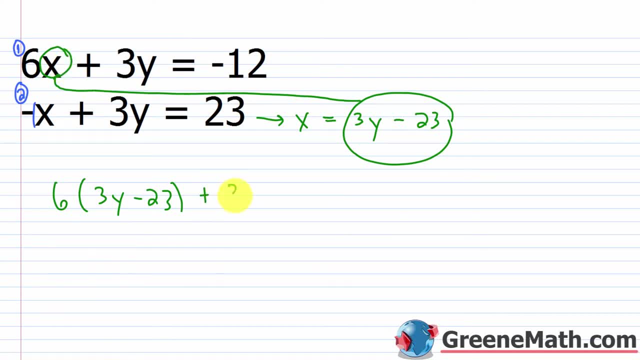 for x there. So once I've done that, then plus 3y equals negative 12.. I have a linear equation in one variable now And it's easy to solve for that variable. So 6 times 3y is 18y And then 6. 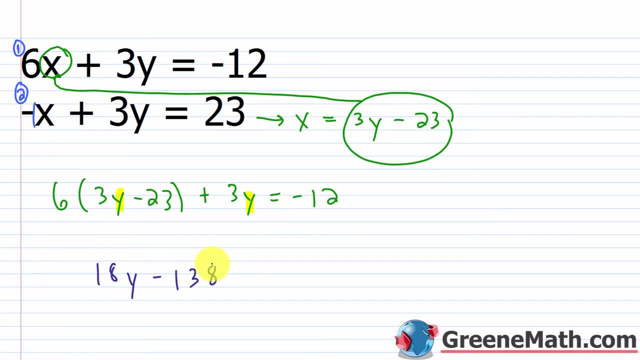 times negative 23 is negative 123.. And then 6 times negative 23 is negative 123.. And then 6 times negative: 138.. And then plus 3y equals negative 12.. So 18y plus 3y is 21y, So I'll have 21y minus. 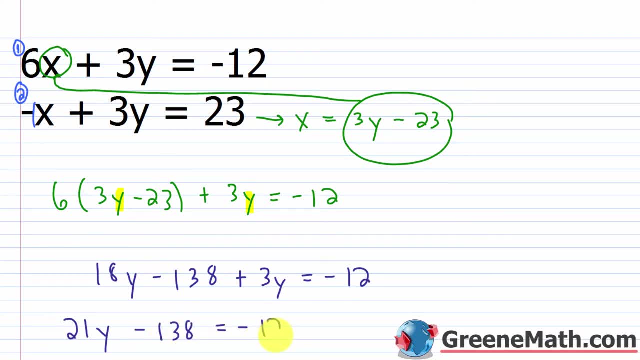 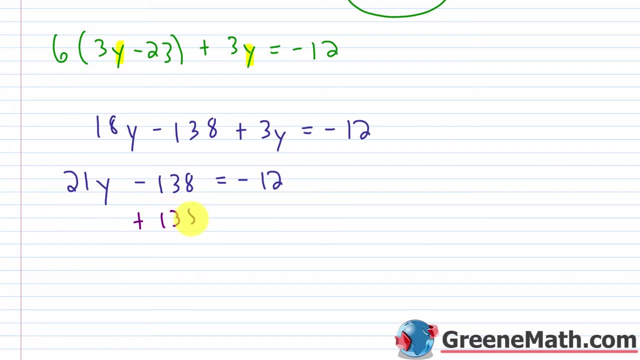 138 is equal to negative 12.. Let's scroll down just a little bit. So now, if I add 138 to each side of the equation, this will cancel And I'll have. 21y is equal to negative 12 times negative. 12 plus 138 is going to be 126.. So as a final step to get y by itself, let's divide both. 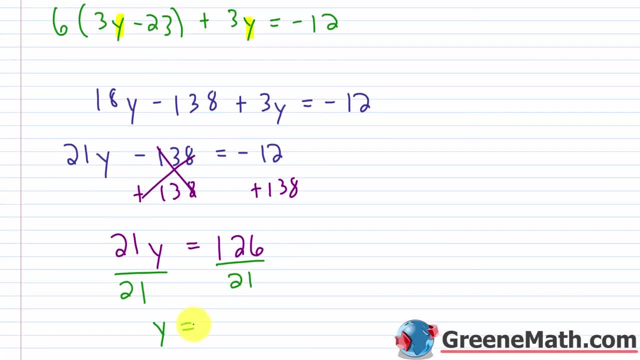 sides of the equation by 21.. And we'll have that y is equal to 6, right 126 divided by 21 is 6.. So y equals 6.. All right, so let's erase everything. So we know that y equals 6.. So the 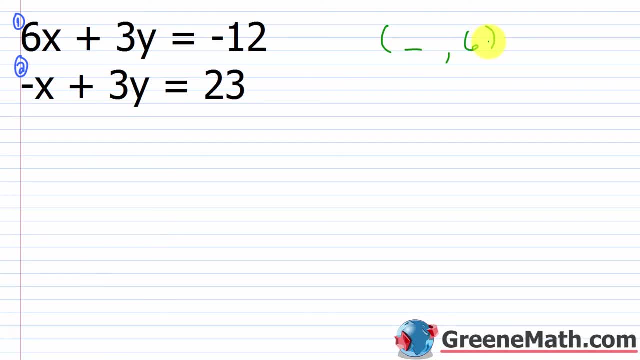 ordered pair would be something comma 6.. So now I can plug in for y in either original equation. Let's go ahead and use our equation. So let's go ahead and use our equation. So let's go ahead and equation 2, because it looks a little easier. So I would have negative x plus 3 times. plug a 6 in for. 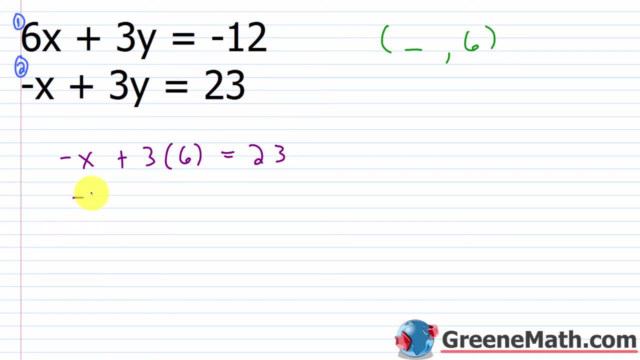 y equals 23.. So negative x plus 3 times 6 is 18, equals 23.. I can subtract 18 away from each side of the equation. This will cancel. I'll have: negative x is equal to 23, minus 18 is 5.. So 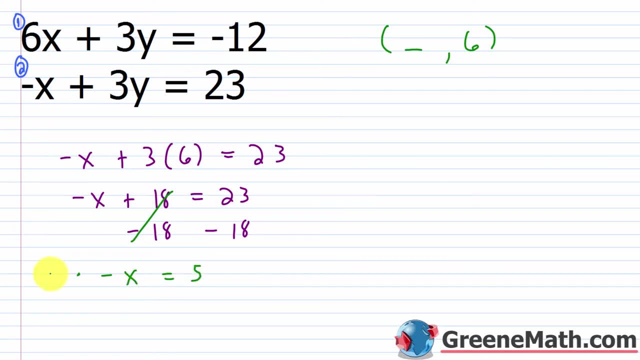 essentially all I need to do is divide both sides by negative 1 or multiply both sides by negative 1. So I'll have negative x plus 3 times. plug a 6 in for y equals 23.. So negative x plus 3 times. 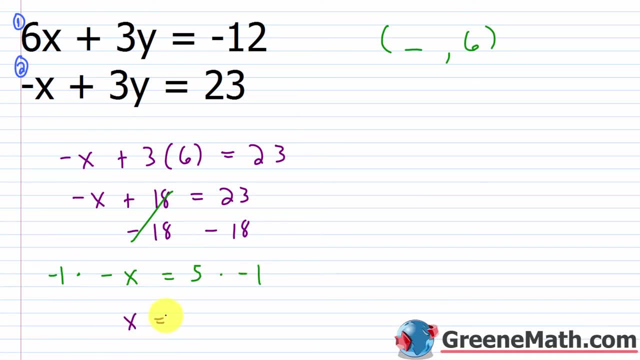 plug a 6 in for y equals 23.. So whatever you want to do, you'll get. x is equal to 5 times negative, 1 is negative 5.. So my x value is negative 5, while my y value is 6.. So the ordered pair negative 5. 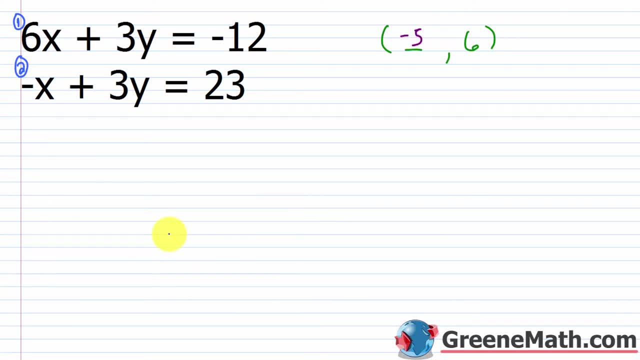 comma 6.. So now what I want to do. I want to go into equation 1 and equation 2, plug in my ordered pair and see if I've got the correct solution for the system. So I've got 6 times for x. 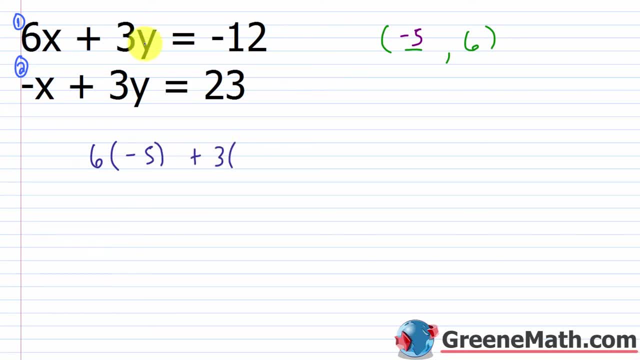 I'm plugging in a negative 5,, plus 3 times for y, I'm plugging in a 6, and this should give me negative 12.. 6 times negative 5 is negative 30, plus 3 times 6 is 18.. This should give me negative 12, and it does right You get. 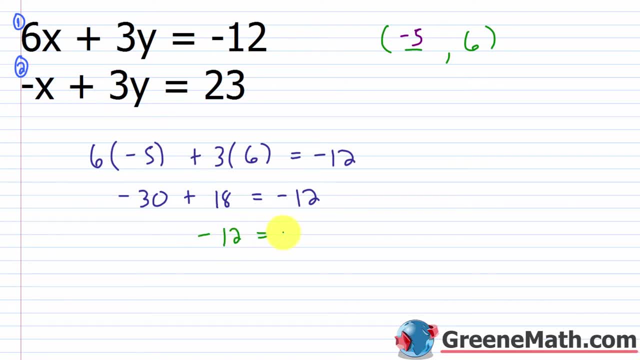 negative 30 plus 18 is negative 12, and that equals negative 12.. So this one checks out. Now for the next one, we have negative and then I'm plugging in a negative 5.. So it's basically the opposite of plug in a negative 5, plus 3 times y, y is 6,. 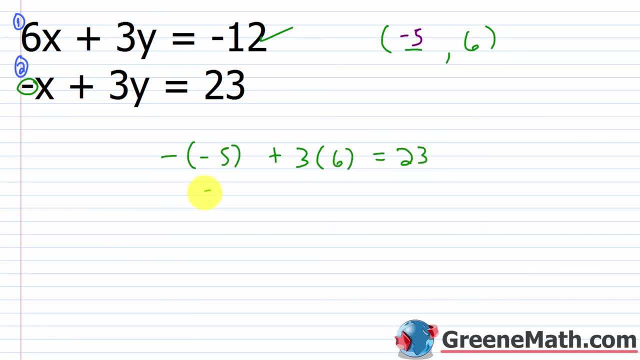 and this should equal negative 12.. So I've got negative 12, and this should give me negative 12.. The opposite of negative: 5 is 5, plus 3 times 6 is 18, and this should equal 23,. and of course it. 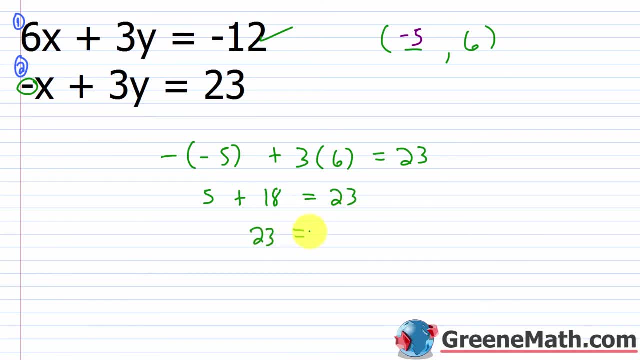 does 5 plus 18 is 23,. so 23 equals 23.. So we verified this one as well. So our ordered pair here, negative 5 comma 6, is the verified solution for this system. All right, so let's take a look. 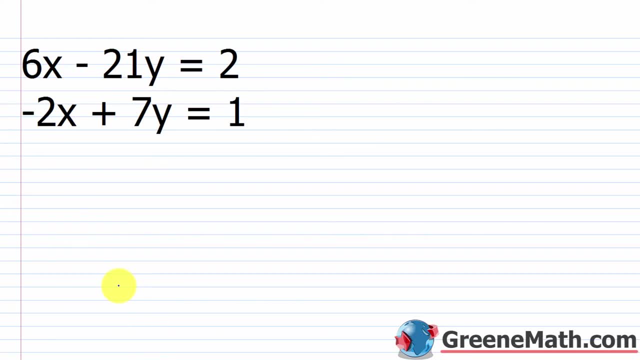 at another one. So we have 6x minus 21y, equals 2.. We have negative 2x plus 7y, equals 1.. So again I'm going to label my equations. This is equation 1,. this is equation 2.. None of the variables have 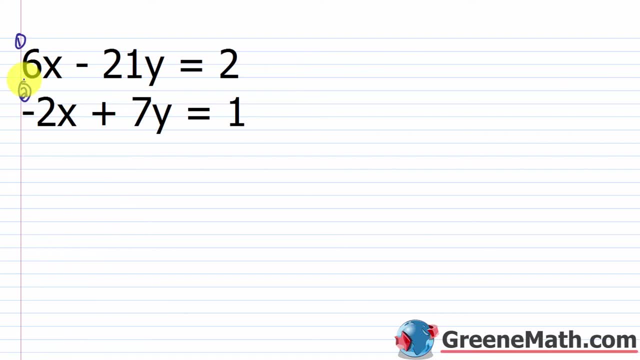 a coefficient of 1,. none of the variables have a coefficient of negative 1.. So pick whatever you want, whatever you think is easiest for you. I'm going to go ahead and solve equation 1 for x, because it's the first thing that I see. So if I have 6x minus 21y equals 2,. 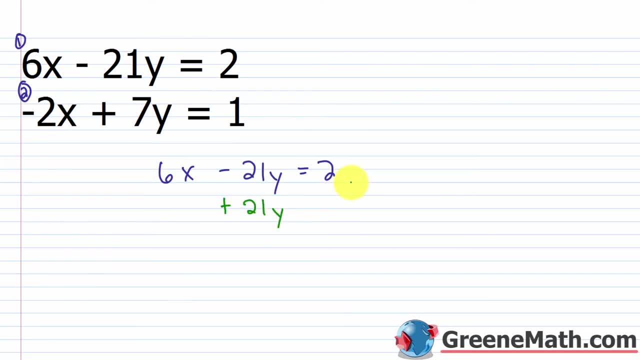 if I'm solving for x, add 21y to each side of the equation. So this is going to cancel. I'll have: 6x is equal to 21y plus 2.. So now I'm going to divide both sides of the equation by 6.. This will. 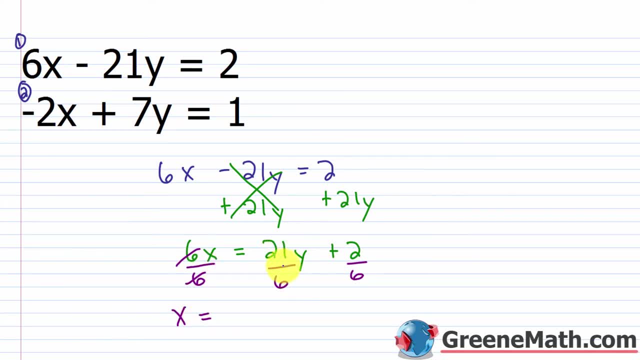 cancel, I'll have. x is equal to for 21 and 6,. they have a common factor of 3.. If I divide 21 by 3, I get 7.. If I divide 6 by 3, I get 2.. So this is 7 halves times y, plus 2 over 6 is 1 third, So x is. 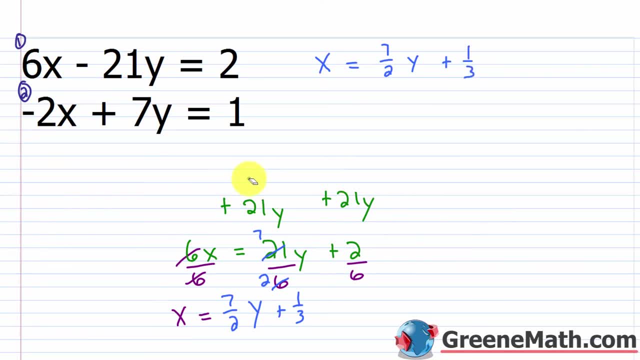 plus 1 third. Okay, so let's erase this. And so we got this from equation 1.. Okay, we got this from equation 1.. So I'm going to plug in for x in equation 2. And I'm going to plug this in. 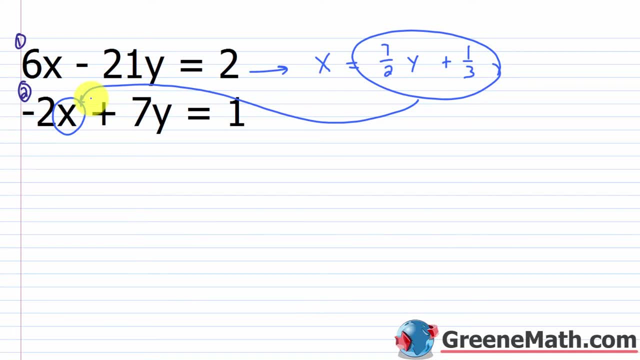 right. x equals this, So that's going in there. So what are we going to get? We're going to have negative 2 times the quantity 7 halves y plus 1 third. then plus 7y equals 1.. So negative 2 times 7 halves. you can think about negative 2 times 7 halves like that. 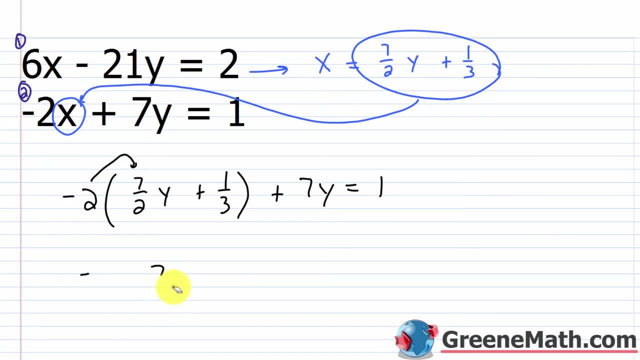 This would cancel with this and you'd have a negative 7.. So this would end up being negative 7y And then negative 2 times 1. third would be negative 2 thirds, And then plus 7y equals 1.. 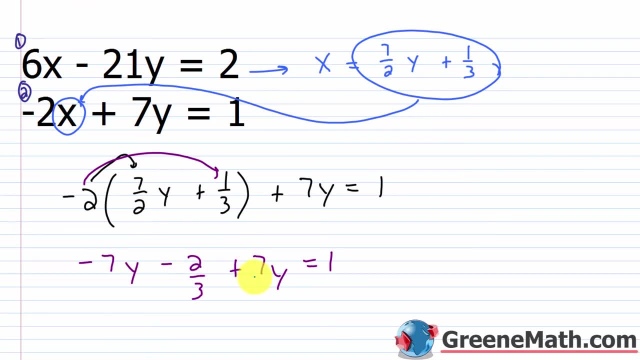 Now what happens here? Negative 7y plus 7y is what That's 0. This cancels. What am I left with? Negative 2 thirds equals 1.. Well, that's not true. That's clearly false. 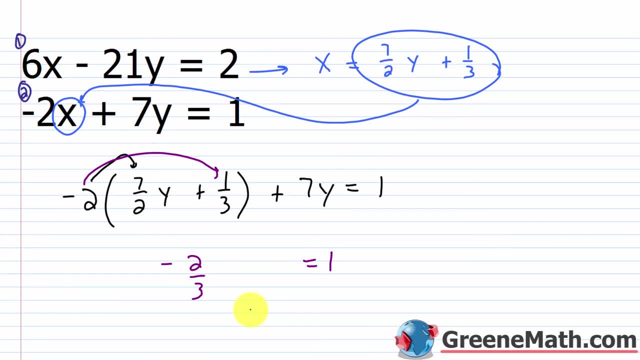 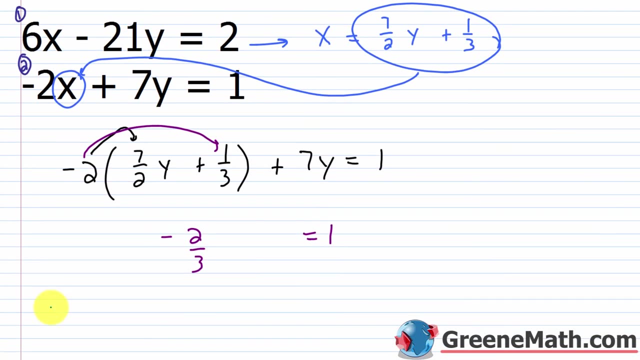 So what happened here? Well, this happens to be a system that has no solution. These are parallel lines, So if your variable drops out when you're doing this and you end up with a statement that doesn't make sense, like negative 2 thirds equals 1, you have no solution. You have no solution. 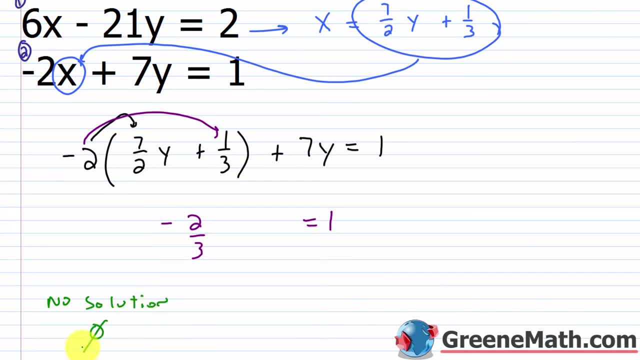 If the variable were to drop out and you have a true statement, then you have an infinite number of solutions. Now the easiest way to show this is again to solve each equation for y. If they're each in slope-intercept form, you can see that they have. 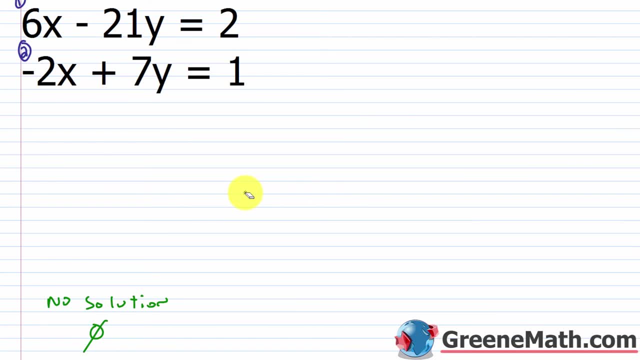 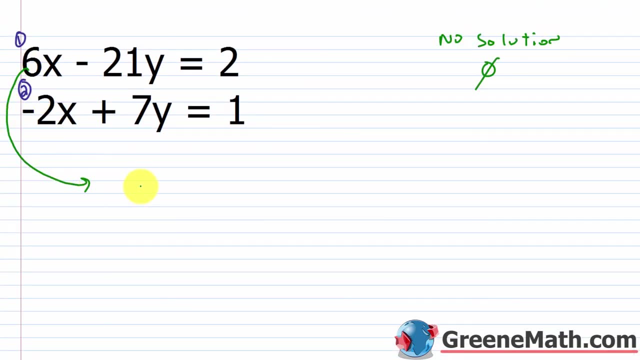 the same slope but different y-intercepts, and so they're parallel lines. So let's put this over here out of the way. If I solve this for y, 6x minus 21y equals 2.. If I subtract 6x away from: 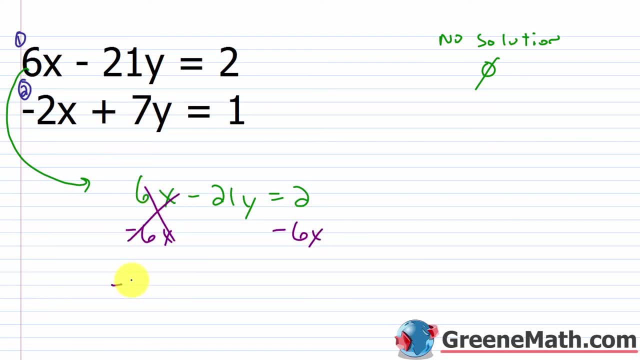 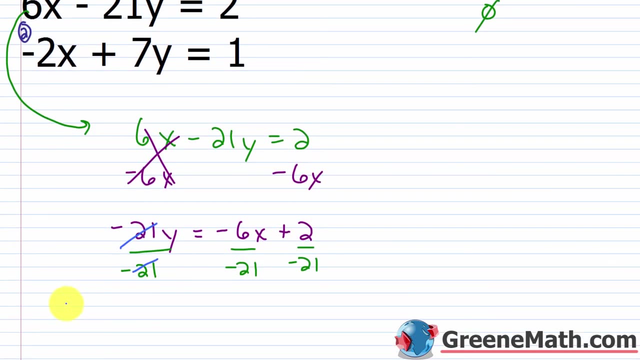 both sides of the equation. this will cancel. I'll have negative 21y is equal to negative 6x plus 2.. I then want to divide both sides of the equation by negative 21.. And so this is going to cancel. I'll have y is equal to. So for negative, 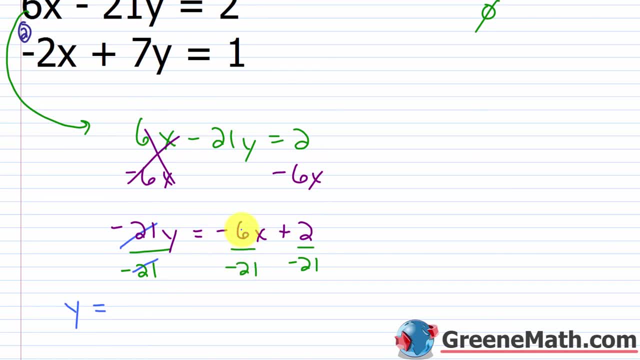 6 over negative, 21, negative over negative is positive, 6 over 21,. they're each divisible by 3.. 6 divided by 3 is 2.. 21 divided by 3 is 7.. Then times x: 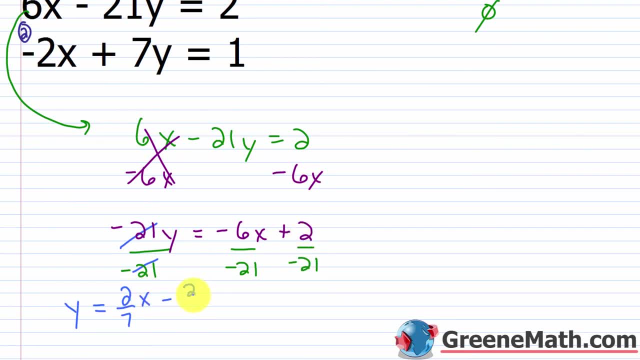 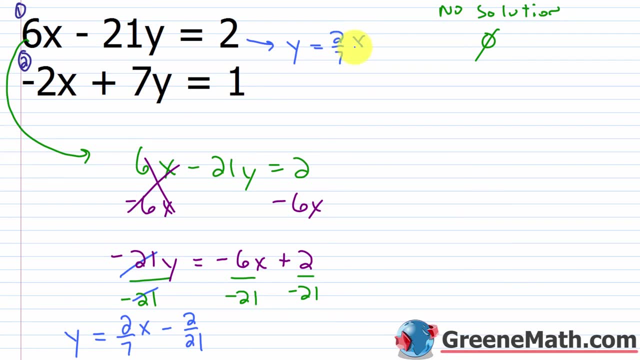 and then 2 over negative 21,. we just write minus 2 over 21.. So that's this guy right here. y equals 2 sevenths x minus 2 over 21.. Okay, Let's erase this and let's now solve this guy for y. 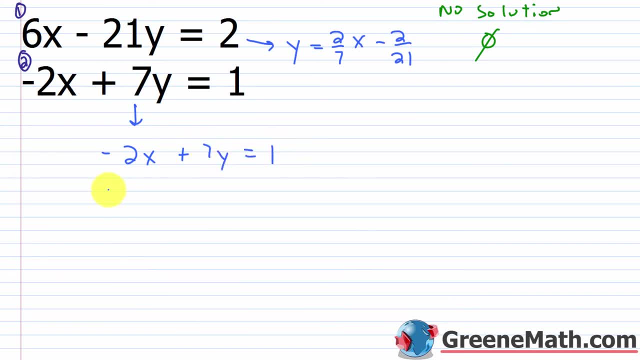 So negative. 2x plus 7y equals 1.. We'll add 2x to each side of the equation, So this is going to cancel. We'll have. 7y is equal to 2y 2x plus 1.. Divide both sides of the equation by 7.. So this cancels. You'll have And I'll. 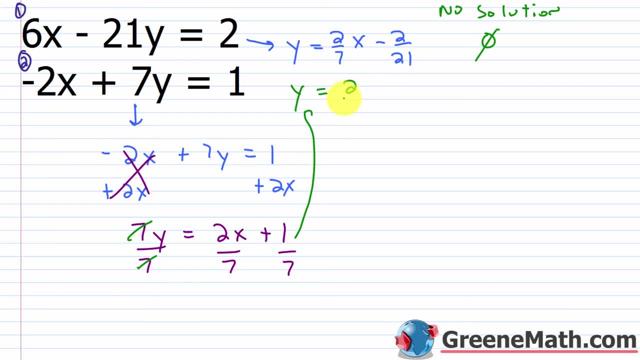 write this up here: y is equal to 2 sevenths x plus 1 seventh. So let me erase this And I want you to look at this real quick. We know that we have parallel lines when what occurs? We have the same slope but different y intercepts. So in this case, the slope, 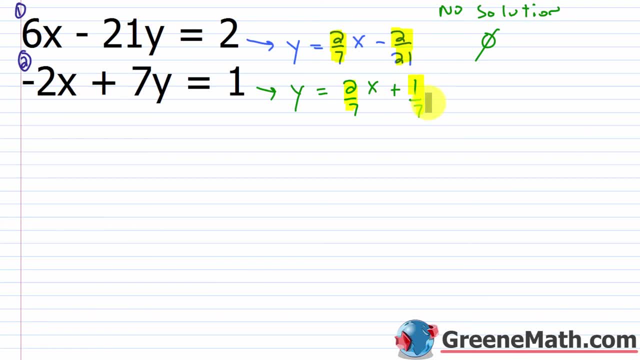 is 2 sevenths for each equation And the y intercepts are different. In equation 1, the y intercept occurs at 0 comma negative 2 over 21.. In equation 2, the y intercept occurs at 0 comma 1 seventh. So same slope, different y intercepts, parallel lines, never going to. 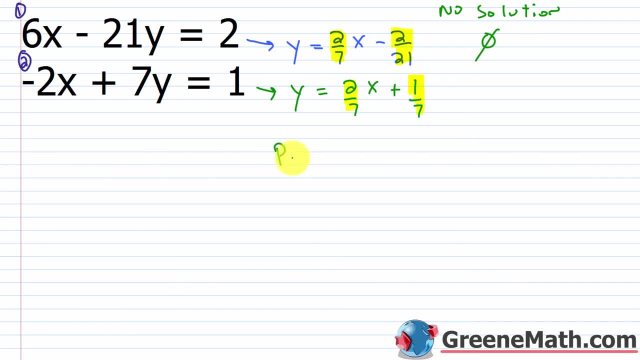 intersect, so there's no solution. Okay, These are parallel lines. All right, Let's take a look at another one. So we have negative 2x minus 2y Y equals 6. And we have 4x plus 6y equals negative 2.. So it looks pretty easy if I solve this guy. 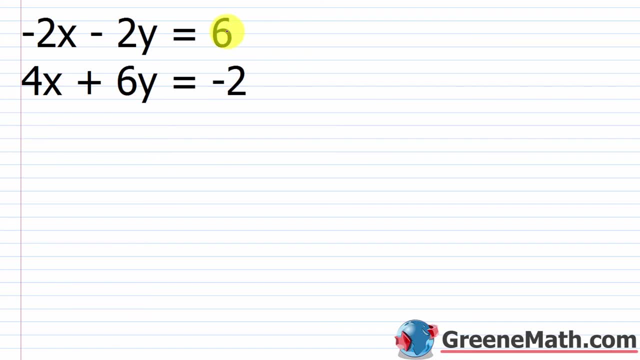 right here for either x or y. That looks easiest to me. So let's label this as equation 1, and this is equation 2.. And I'll go ahead and solve equation 1 for, let's say, x, So negative 2x minus 2y. 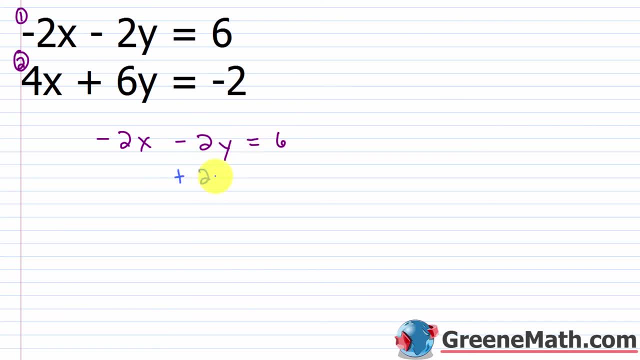 equals 6.. Let's go ahead and add 2y to both sides of the equation. That'll cancel. We'll have negative. 2x is equal to 2y plus 6.. And as a final step, let's divide both sides of the equation by. 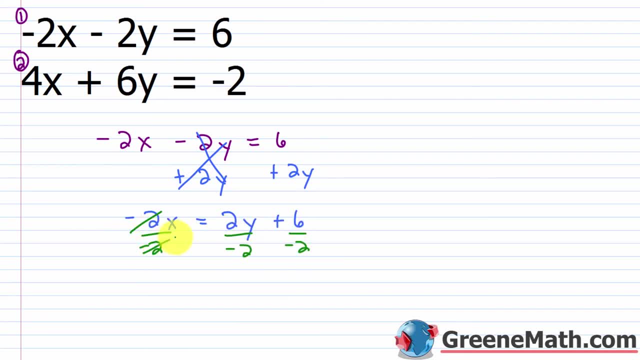 negative 2.. So that'll cancel. I'll have: x is equal to 2 over negative, 2 is negative 1, so negative y. 6 over negative 2 is negative 3, so minus 3.. So x is equal to negative y minus 3.. 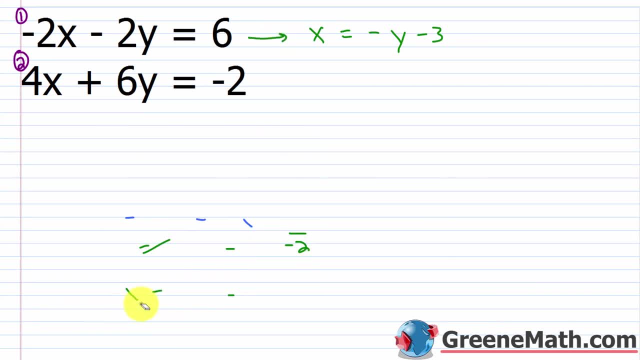 So now what am I going to do? I'm going to plug in 4x in equation 2. now I found out that x is equal to, or x is the same as, negative y minus 3, that quantity. So I can plug in for x in the second equation So 4 times again this quantity here. 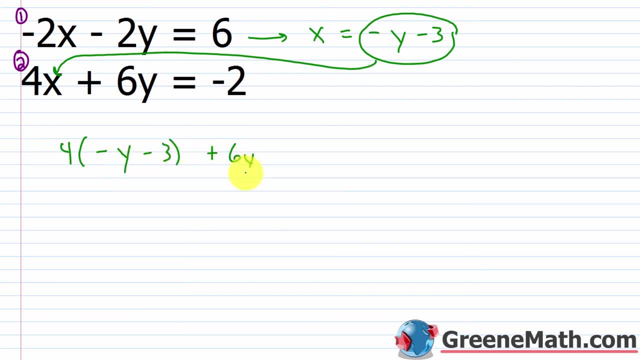 negative y minus 3, then plus 6y is equal to negative 2.. All right, so 4 times negative y is negative 4y. 4 times negative 3 is minus 12, then plus 6y equals negative 2.. 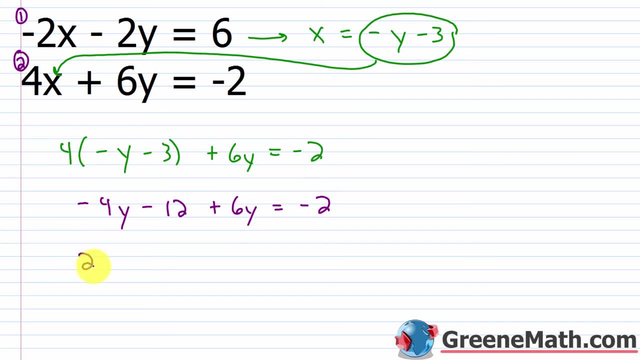 All right. so negative 4y plus 6y is 2y. then minus 12 equals negative 2.. And again, if I add 12 to both sides of the equation, that will cancel, We'll have: 2y is equal to negative. 2 plus 12 is. 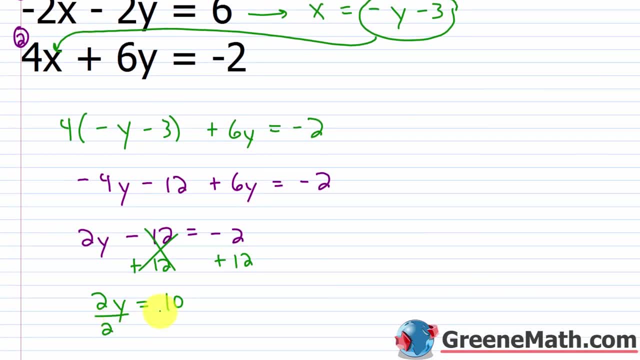 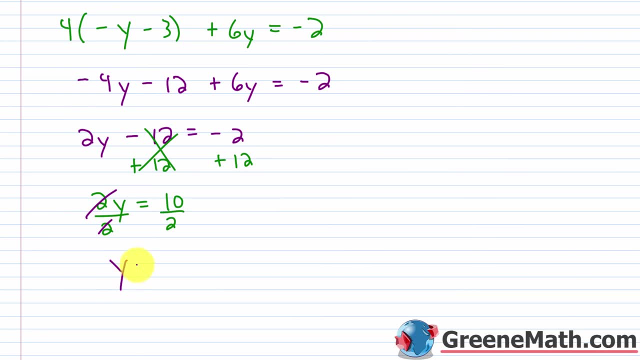 10.. As a final step, I'm going to divide both sides by 2, and we're going to get that. I'm going to scroll down a little bit. We're running out of room, So this will cancel. y is equal to. 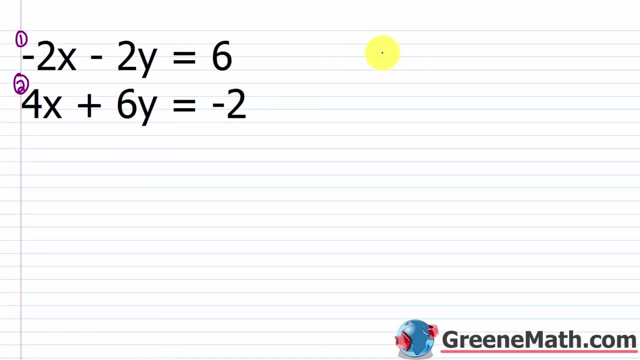 5. Let's erase everything. So we say that y equals 5.. So as an ordered pair, something comma 5.. All right, so I'm going to plug in for y in either original equation, Equation 1 or 2, doesn't. 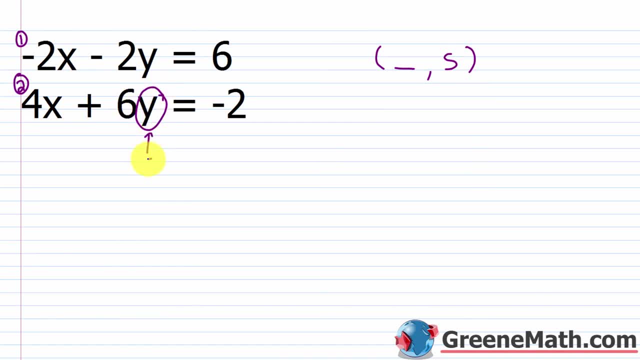 matter. Let's go ahead and pick equation 2.. So I'm going to plug in a 5 there. So I would have 4x plus 6 times 5 is 30.. So plus 30 equals negative 2. So let's subtract 30 away from each side of. 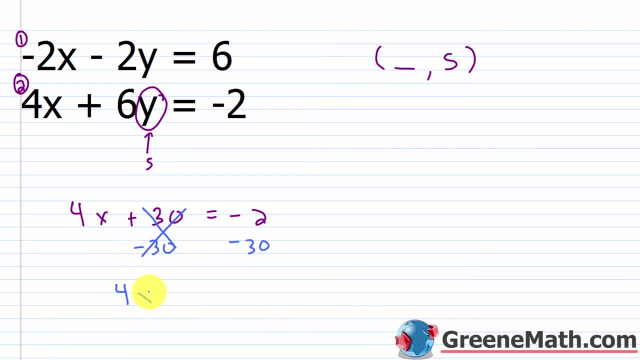 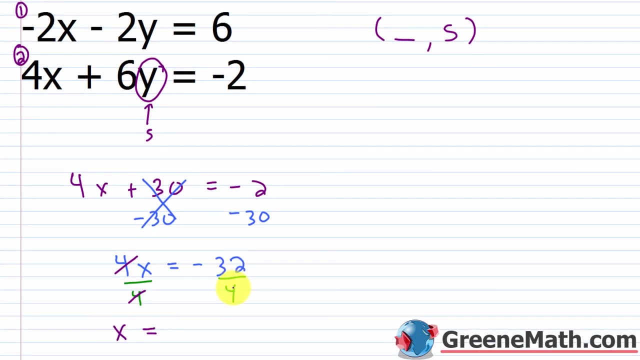 the equation. This would cancel. 4x is equal to negative, 2 minus 30 is negative 32.. As a final step, let's divide both sides by 4.. And this is going to cancel. We're going to end up with: x is equal to negative, 32 over 4 is negative 8.. So my 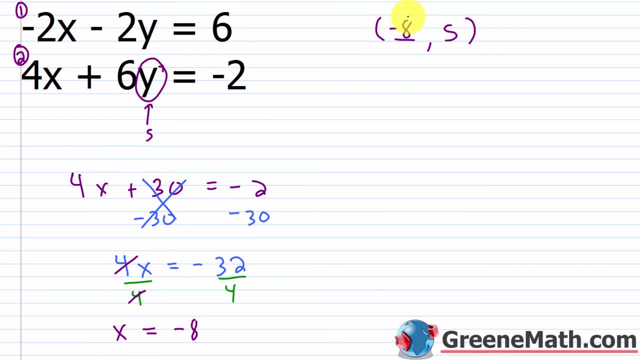 x value is negative 8.. My y value is 5.. Or again the ordered pair, negative, 8 comma 5.. So let's check this. I'm going to go ahead and plug into each original equation. So in equation 1, I have 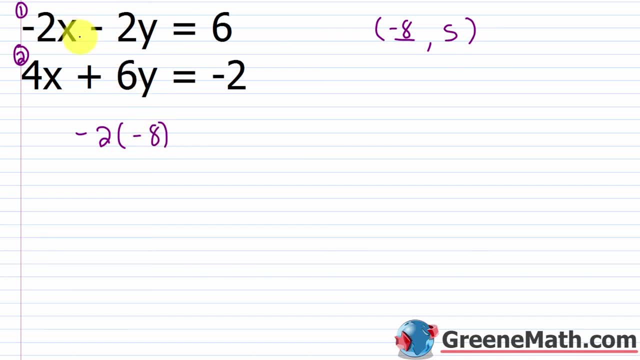 negative 2 times negative 8.. That's my value for x Minus 2 times 5.. That's my value for y, And this should equal 6.. Negative 2 times negative, 8 is 16.. Negative 2 times 5 is: 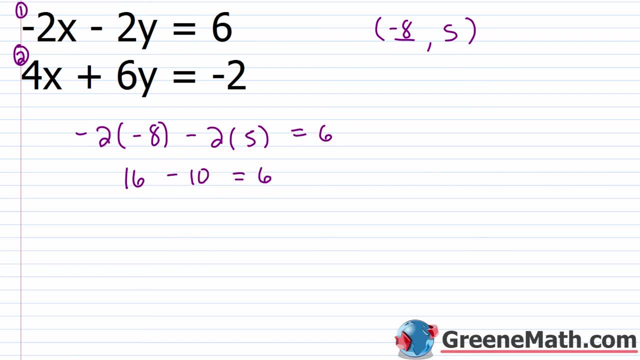 negative 10. And then we have equals 6. So 16 minus 10 is 6.. So you get 6 equals 6.. So it works out here In the second equation- remember that's what we use to find x. We know it already works. 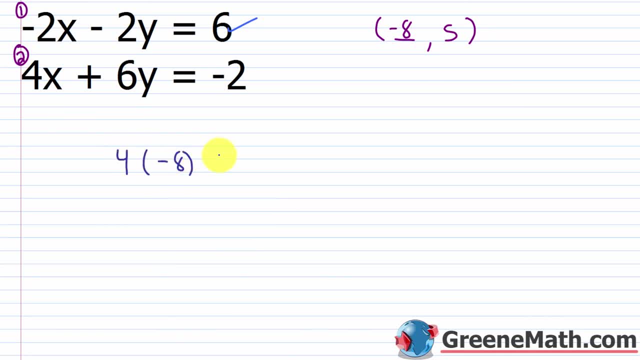 Substitute it anyway. 4 times we have negative 8 for x, plus 6 times we have 5 for y. this should equal negative 2.. 4 times negative 8 is negative 32, plus 6 times 5 is 30,. this should equal negative. 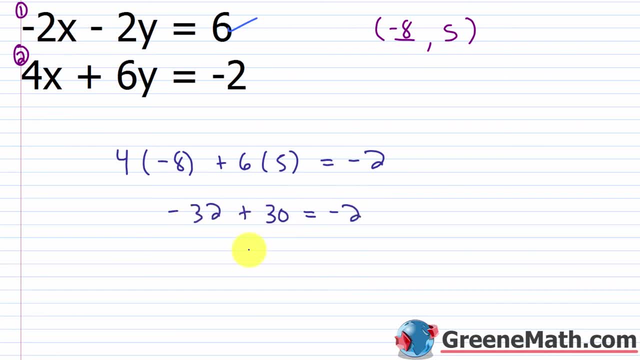 2, and of course it does Negative. 32 plus 30 is negative 2, so negative 2 equals negative 2.. So it works out here as well. So we've verified that the ordered pair negative 8 comma 5, is our solution for this system. 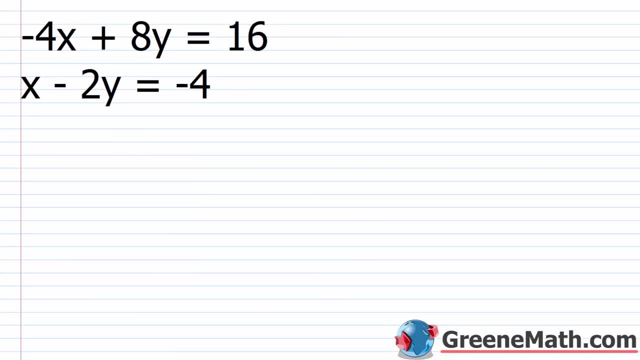 Alright, let's take a look at one more problem. So we have negative 4x plus 8y equals 16, and we have x minus 2y equals negative 4.. So I notice that this equation here- and I'm going to label this equation 1 and equation 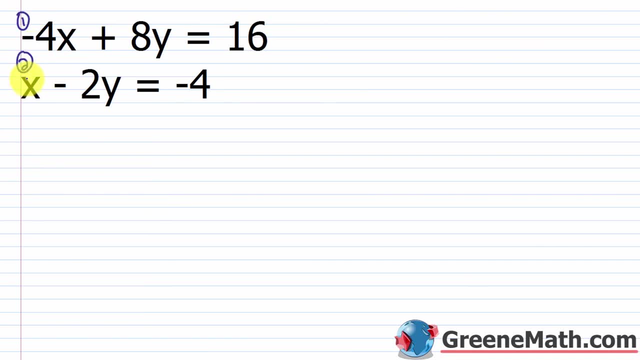 2, this equation 2 has a coefficient on x, that is 1.. So when that occurs, it's like hitting the lottery. right, You want to solve for that one. I've got to use that because it's easy, So I'm going to say: okay, I have x minus 2y equals negative 4.. 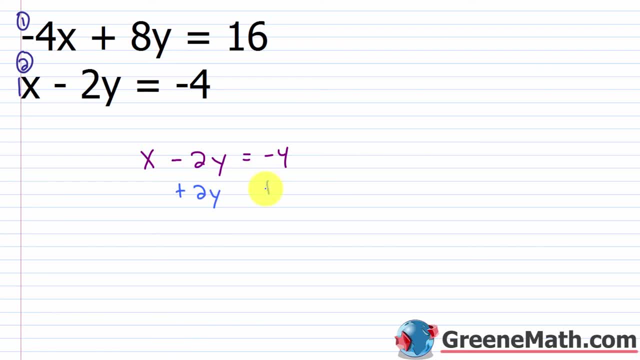 I'm going to add 2y to both sides of the equation. This will cancel. We'll have: x is equal to 2y minus 4.. So now if I know what x equals or what x is, the same as I can plug in for x in equation. 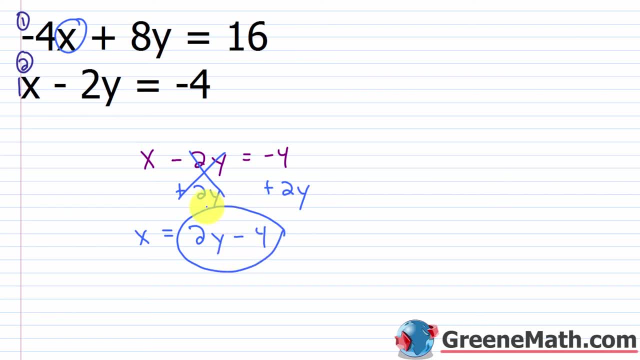 1. So I'm going to plug this quantity 2y minus 4, in for x there. So I would have what I would have: negative 4 times the quantity 2y minus 4.. So I'm going to plug this quantity 2y minus 4, in for x there. 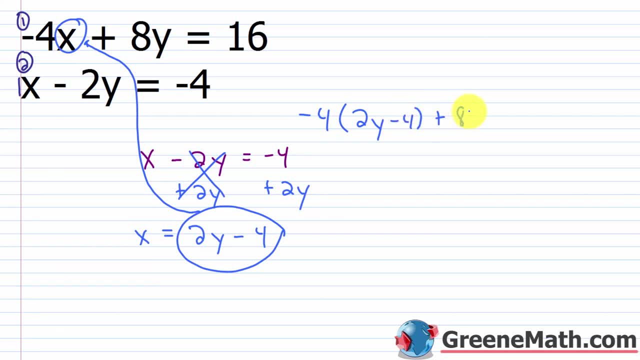 So I would have what I would have: negative 4 times the quantity 2y minus 4, plus 8y equals 16.. So let me kind of do this off to the side here. Negative 4 times 2y is negative 8y. 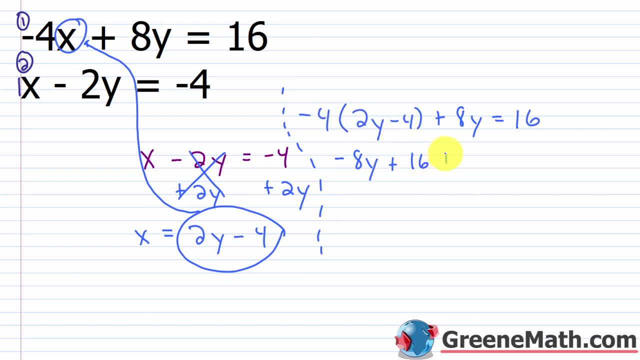 Then negative 4 times negative 4 is plus 16.. Then plus 8y equals 16.. Negative 8y plus 8y is 0.. This cancels, Uh-oh, my variable dropped out again. So I have what. 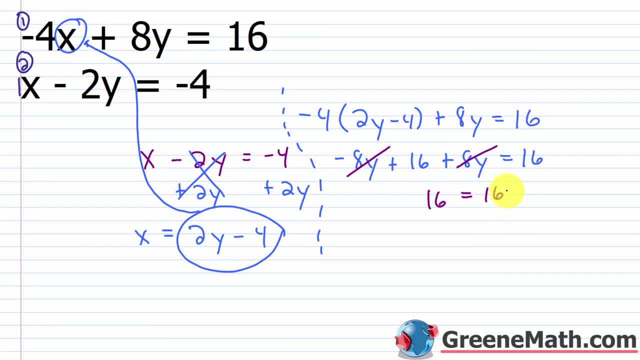 I have 16 equals 16.. Or if I subtract the 16 away from each side of the equation, I'd have 0 equals 0. So what I told you when we had that example? with no solution If the variable drops out and you're left with a true statement. 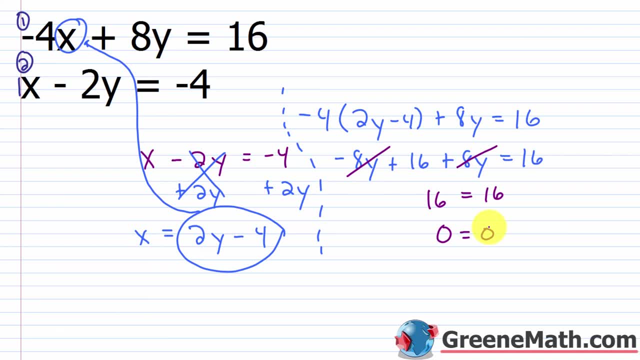 Like you are here, You have an infinite number of solutions. You basically have the same equation for equation 1 and 2. It's just algebraically manipulated to look different. So let's just write that We have an infinite number of solutions. 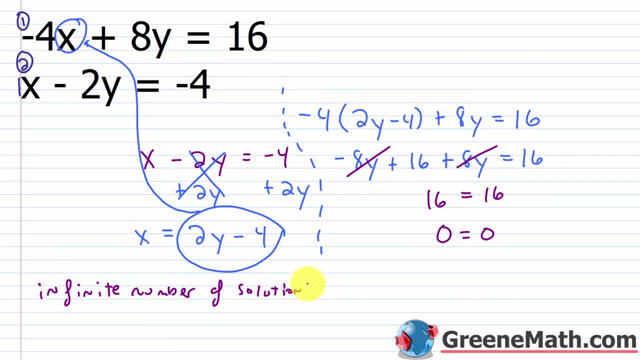 Okay, So We have an infinite number of solutions. How could we prove that these two equations are the same? There's a number of different things we could do. The easiest thing you could do is look at it and say: well, if I multiply this right. 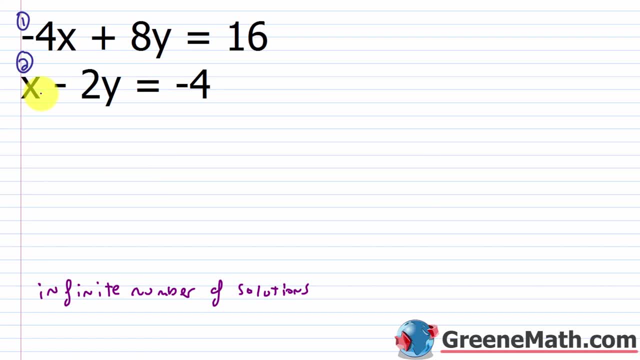 here equation 2 by negative 4 on both sides, I would get equation 1. So negative 4 times, the left side is x minus 2y, The right side is negative 4. So multiply that by negative 4 as well. 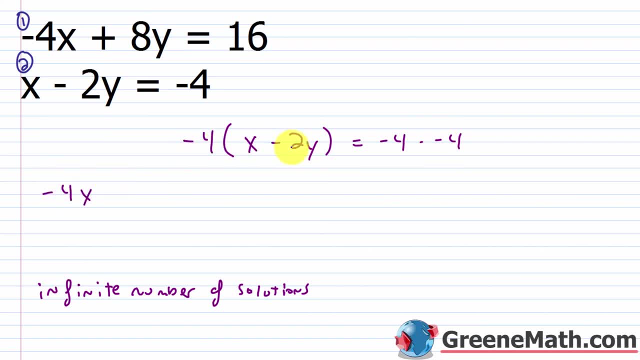 So negative 4 times x is negative 4x. Okay, Negative 4 times negative. 2y is plus 8y. This equals negative 4 times negative. 4 is 16.. So now I took equation 2.. I multiplied both sides by the same non-zero value. 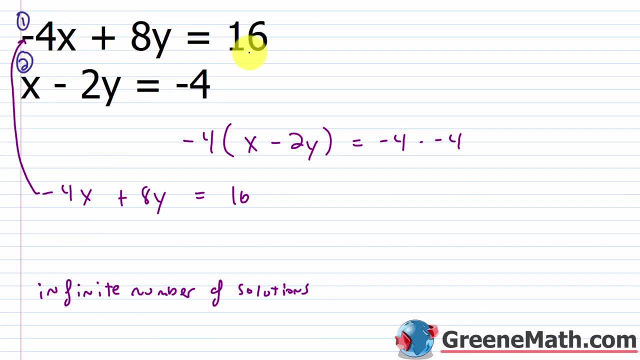 And I came up with equation 1. Negative 4x plus 8y equals 16. Negative 4x plus 8y equals 16. So it's the same equation. Now, the other thing we could do is we could solve each equation for y. 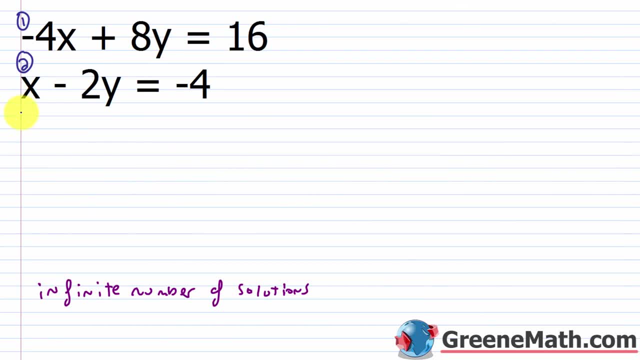 And again you'd see that you have the exact same equation. So if I subtract x away from each side of the equation Here I'd have: negative 2y is equal to negative x minus 4.. Divide both sides by negative 2.. 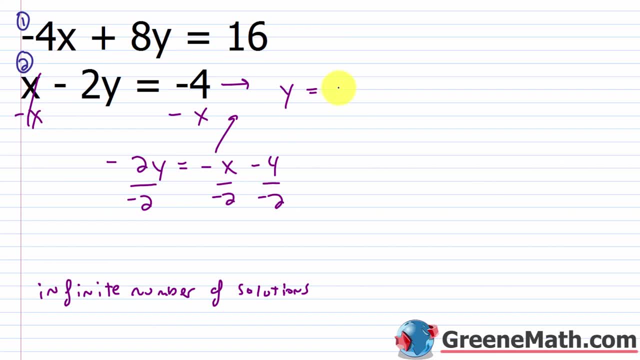 So that would give me: y is equal to negative over negative is positive. So one half times x negative, 4 over negative, 2 is plus 2.. Now for this one up top: if I have negative, 4x plus 8y equals 16.. 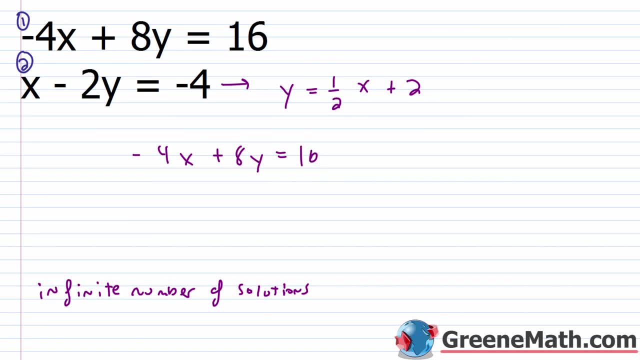 Okay, Okay, Negative 4x plus 8y is equal to negative 4x plus 16.. I would add 4x to both sides of the equation. I would cancel. I'd have: 8y is equal to 4x plus 16..